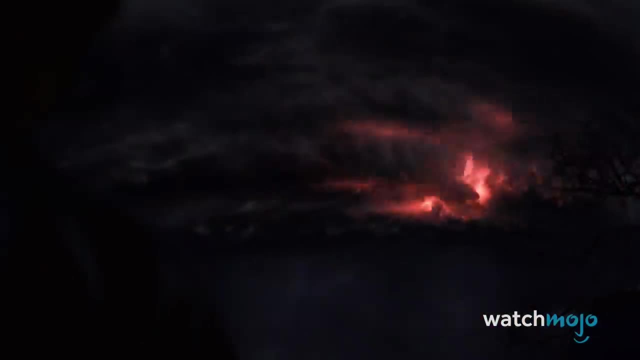 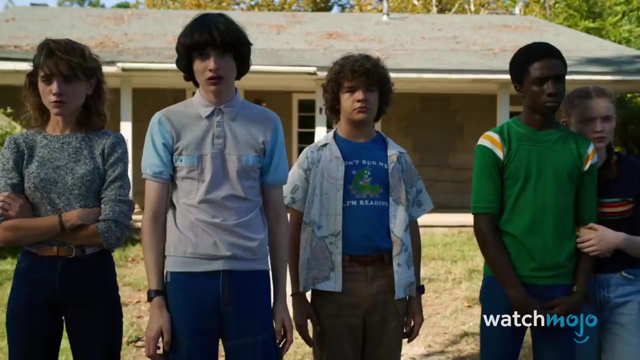 That being said, the six-figure salaries of the ensemble probably eat up a big chunk of change too. All right, you want a scoop of chocolate? That's $1.25.. Still, the investment has paid off big time, given Stranger Things' popularity. 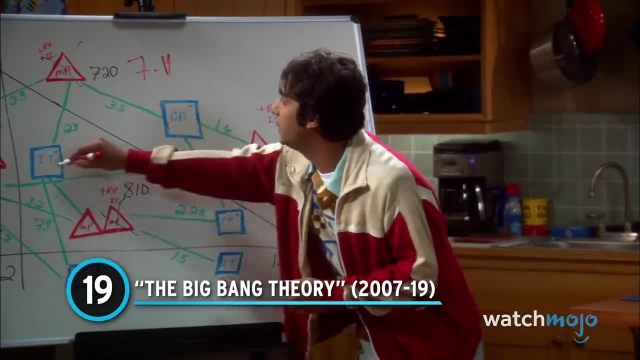 Number 19, The Big Bang Theory. The Big Bang Theory is an TV series that is a hit in the world as a whole. The show stars a number of male and female characters and shows an amazing acting. Sitcoms are generally cost-effective to produce, but there are a few expensive ones out there. The Big Bang Theory started off modestly, but given that it ran for 12 years and ranked among TV's most-watched shows, for many of them, the show could afford to invest in itself. A big part of these rising costs were the stars' salaries. By the later seasons, the original core cast members were making a million dollars per episode, and though that eventually dropped to $900,000, that was only to help bridge the gap with their co-stars Mayim Bialik and Melissa Rauch, who were each earning a reported. 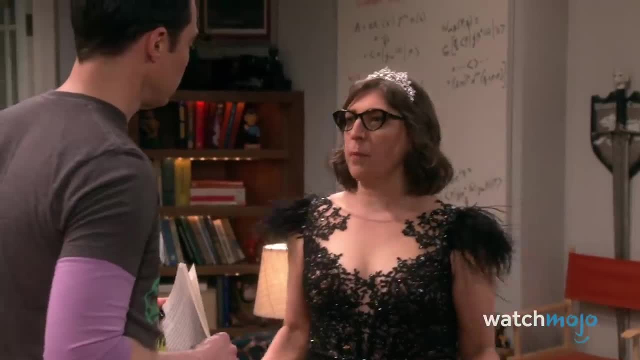 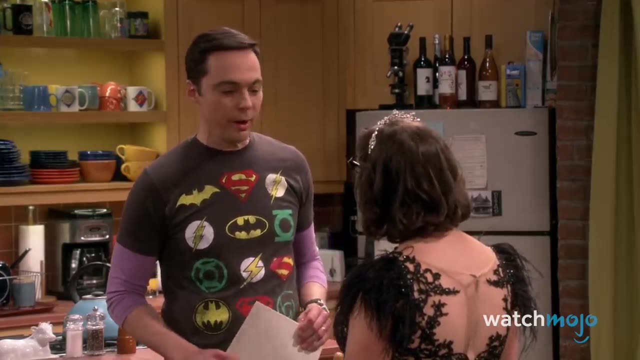 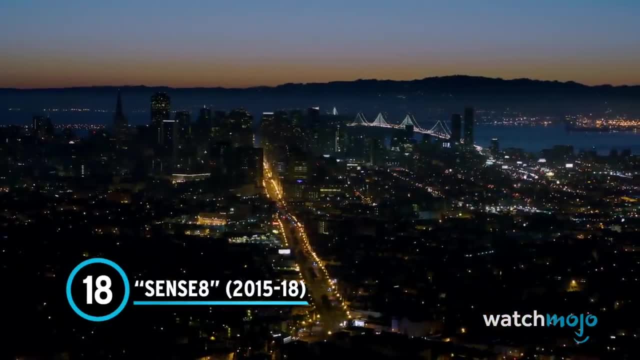 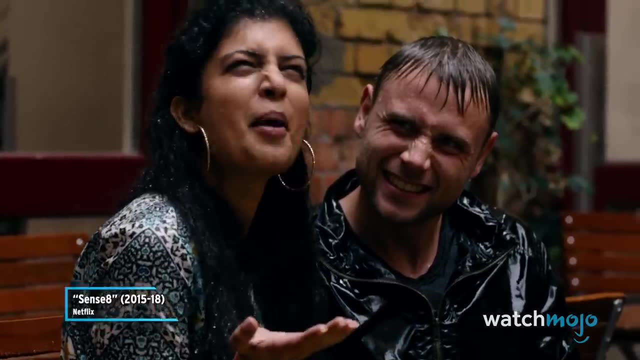 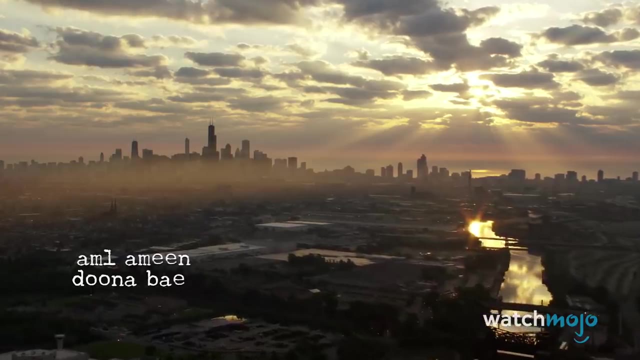 Number 18, Sense8.. Sense8 follows a group of eight disparate people from around the world who discover they're psychologically and emotionally connected. It seems like it's in Bombay, but it's not so cold. A truly global series. the show was shot in 13 different countries. 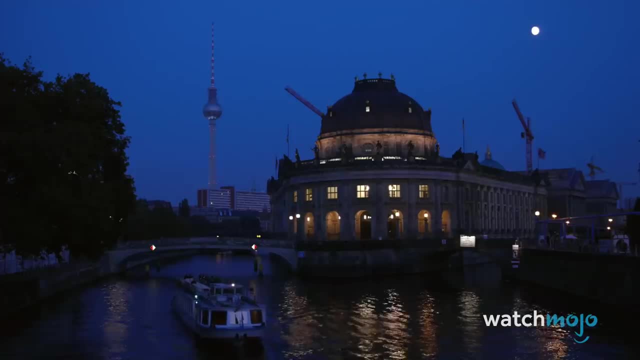 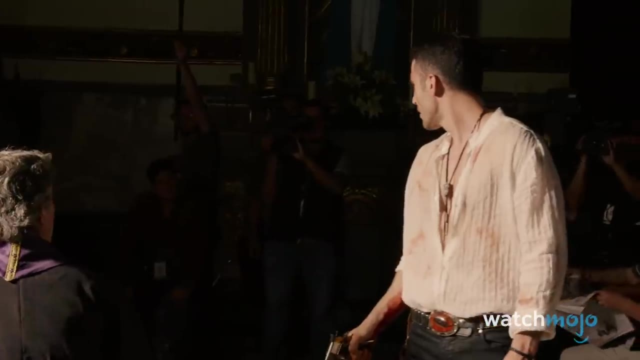 Location shooting can get expensive and Sense8 racked up a hefty budget to make the show a hit. The show was a success with a budget of $9 million per episode for its second season. Ironically, despite being about connection, Sense8 failed to connect with a wide enough. 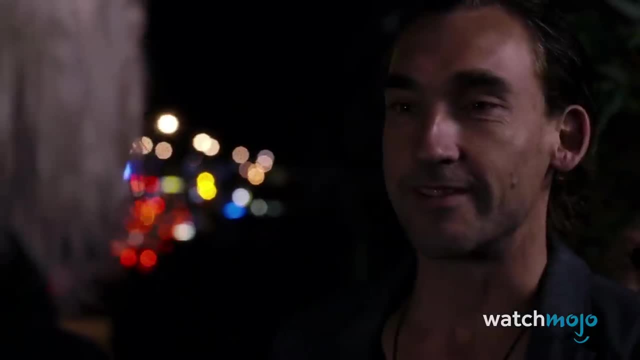 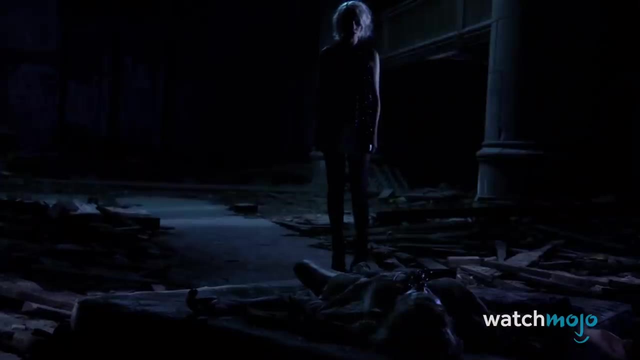 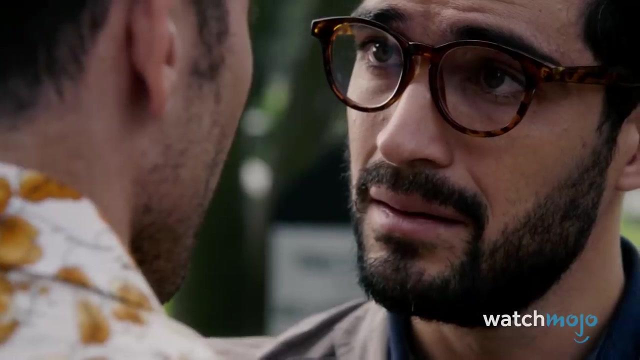 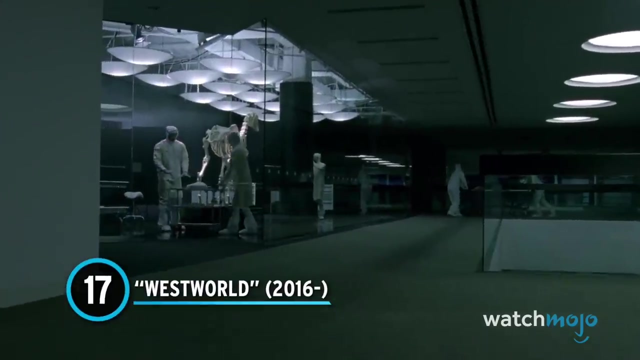 audience. This likely contributed to Netflix's decision to cancel it. No matter how groundbreaking or good a show is, a network won't shell out that kind of cash if they aren't seeing a solid return on investment. Number 17, Westworld. 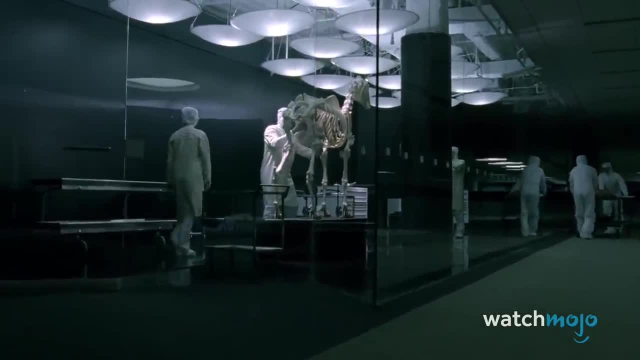 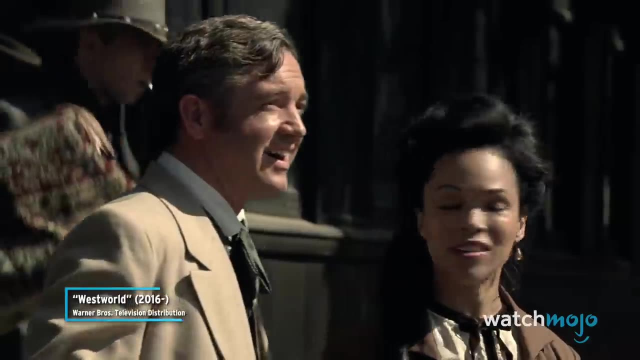 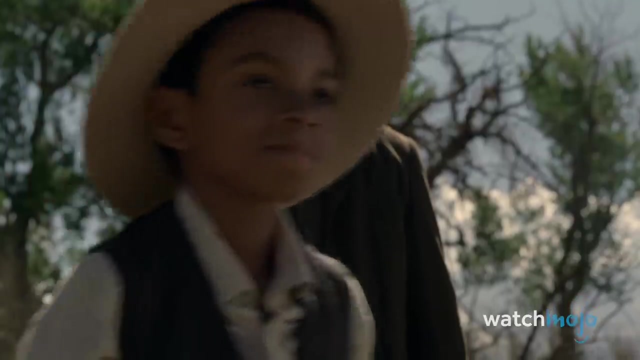 These violent delights come at a cost. Sci-fi shows and period dramas tend to ring up TV's highest budgets, and Westworld is basically both at once Set in the future, where the wealthy pay to experience a realistic simulation of the Old West and other locales. Westworld is visually stunning. Amazing locations and fantastic effects, and of course, it has an A-list cast which cannot be easy on the wallet. According to The Hollywood Reporter, the show's first season cost between $8 to $10 million for each episode. Season 2 and 3 are said to have cost over $100 million apiece. 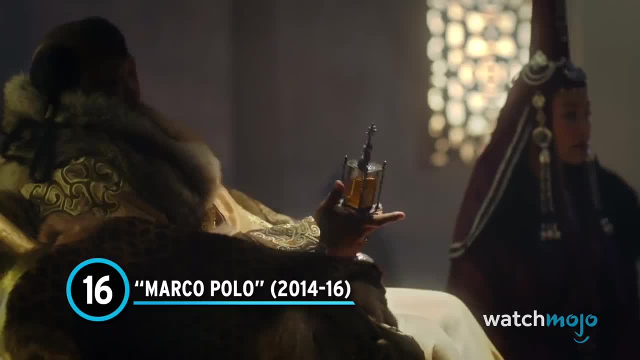 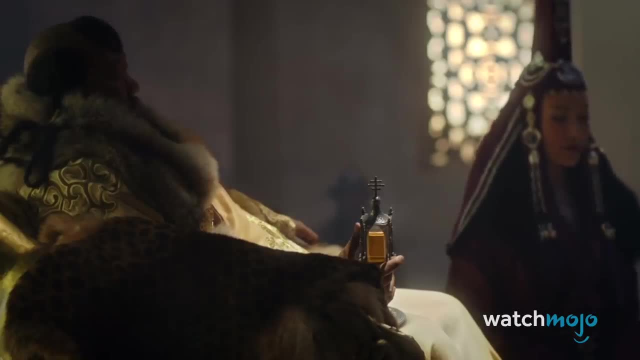 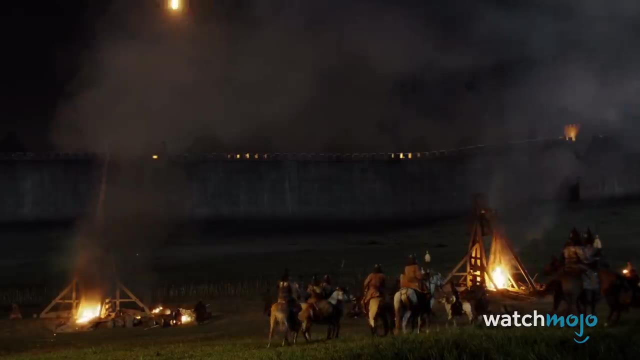 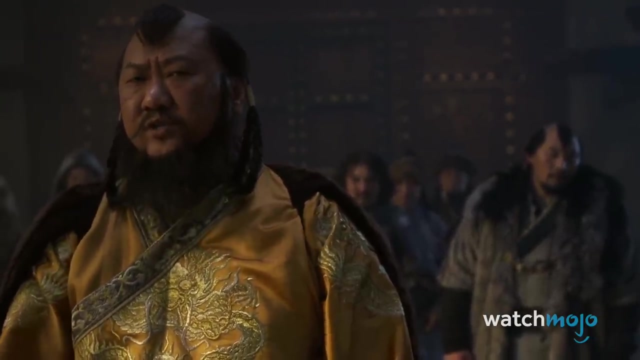 Number 16, Marco Polo. Here's a Netflix original that wasn't successful enough to justify the huge amounts of cash spent on it. The historical drama about its titular explorer required lavish sets and costumes to recreate the period setting of late 13th century China, which resulted in Netflix paying $90 million. 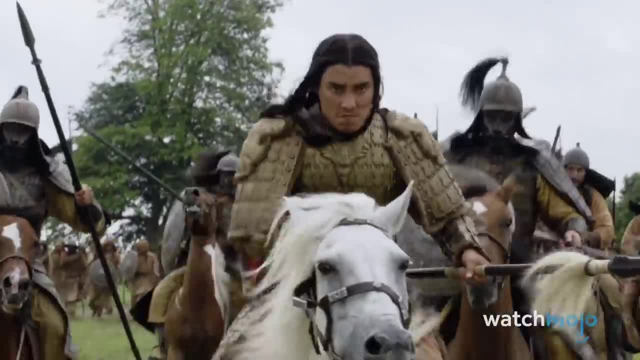 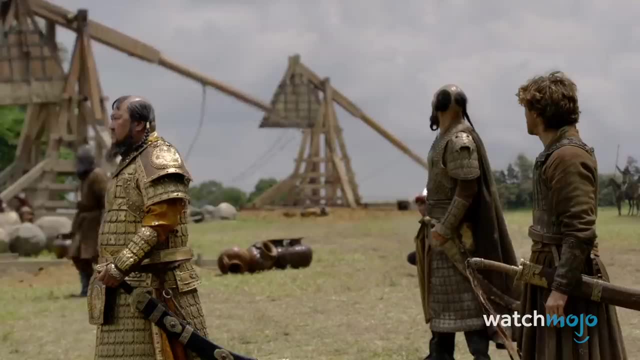 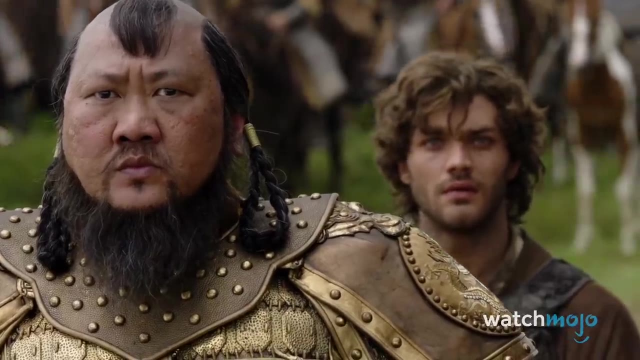 for the entire series, A huge number for any TV show. Unfortunately, the series debuted to middling reviews and, while it made it to a second season, Marco Polo's journey ended shortly after that. Thankfully for Netflix, this poor investment is more an exception than the rule. 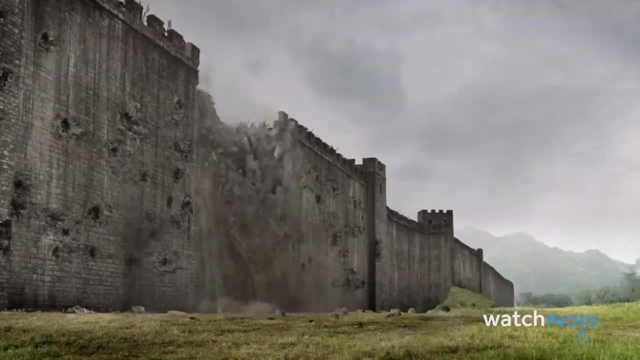 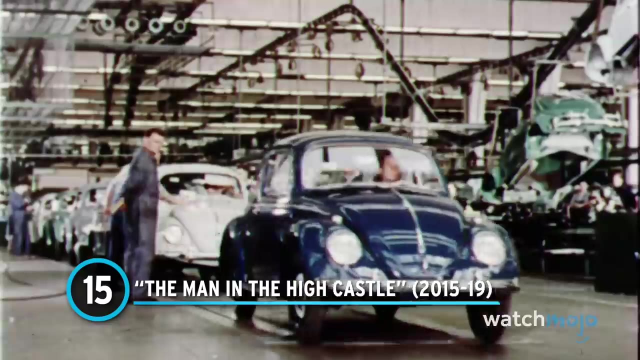 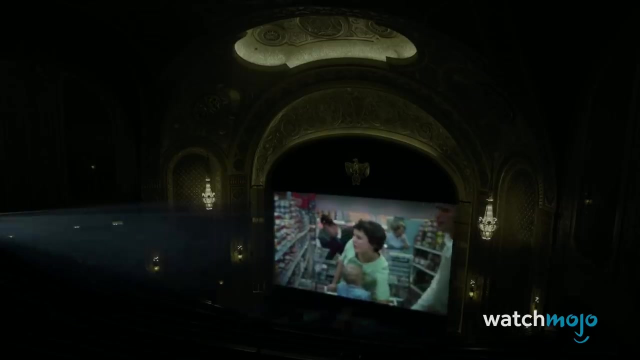 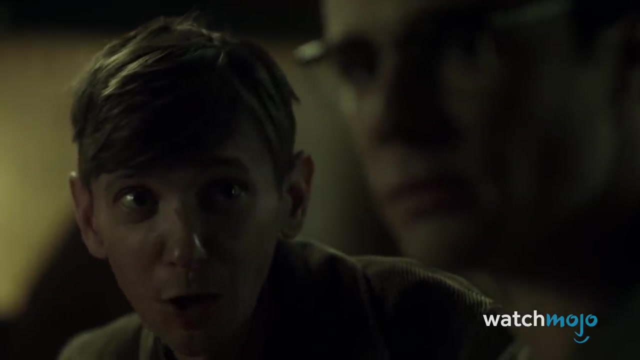 Number 15. The Man in the High Castle, An Amazon original series. The Man in the High Castle is set in the 1960s, in a parallel world where the Axis powers won the Second World War. As we've stated, period pieces tend to be costly. 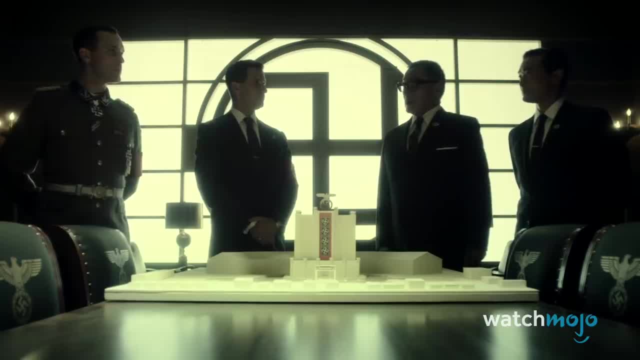 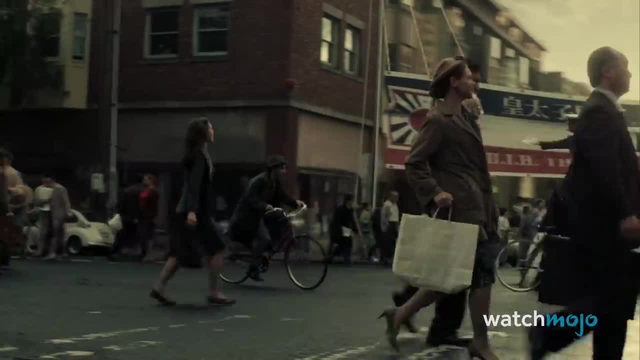 as the sets, costumes and props all have to be era-appropriate. I'm sorry, The furniture in this room is inappropriate for the Crown, Prince and Princess. The Man in the High Castle has to convincingly create an alternate history with all of the above. plus special effects. According to reports, the show required around $10 million each episode to pull it off- An excellent price. Sadly, despite a strong start, the show's high budget wasn't enough to maintain high enough viewing numbers to keep it going beyond four seasons. 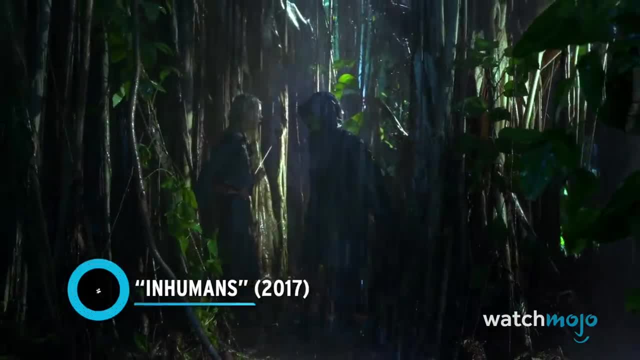 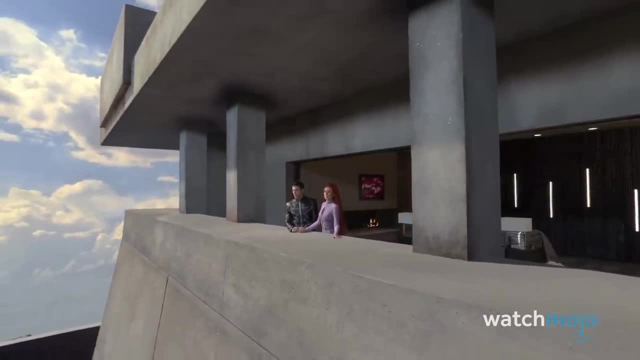 Well, it was only a matter of time before we got to a Marvel property. What are we? We are Inhumans. Inhumans had quite a bit of buzz before its release, as the series was partnered with IMAX, which paid for the first two episodes. 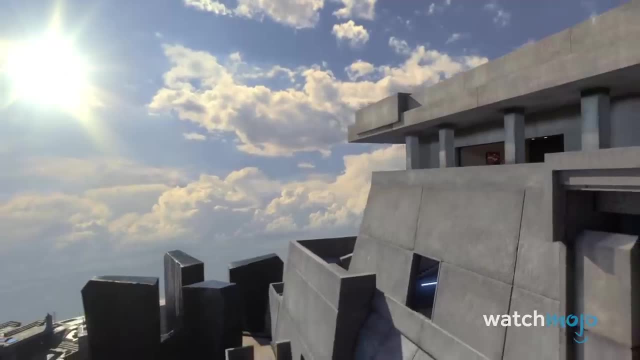 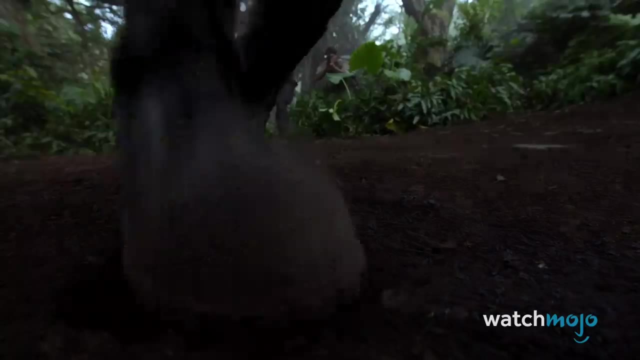 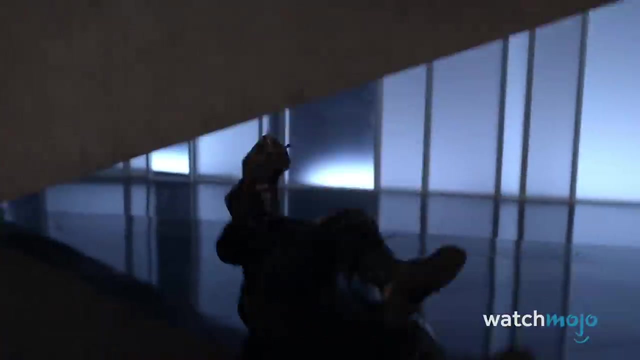 The short series is estimated to have budgeted as much as $8 to $10 million towards each of its eight episodes, Never approach downwind dumbass. Still, it's odd that one of the most expensive shows in Marvel's extensive cinematic universe thus far 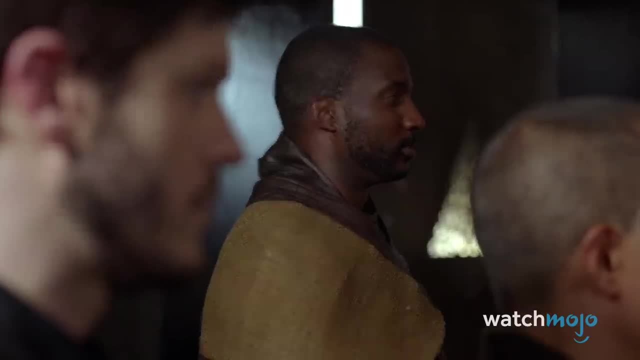 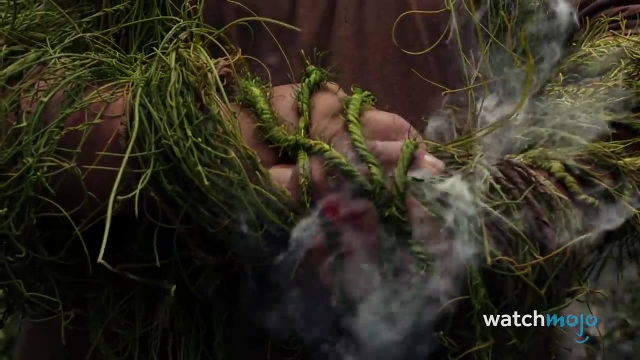 is also one of its least successful. None of it matters in the long run. Eventually, the universe will grow darker until black holes dominate the cosmos, But some factors, like the short shooting schedules and a lack of engaging characters, serve as a reminder that there are some things that money cannot fix. 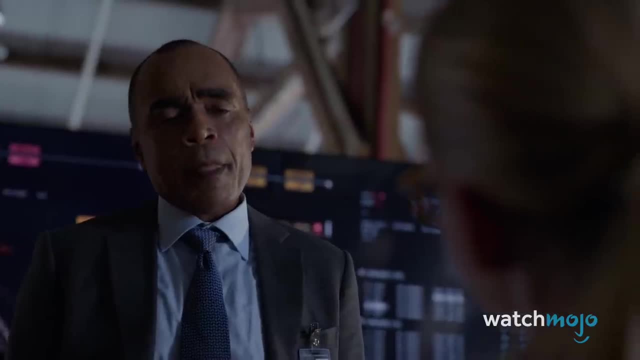 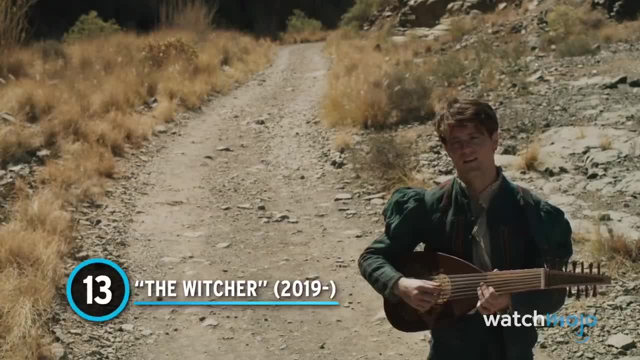 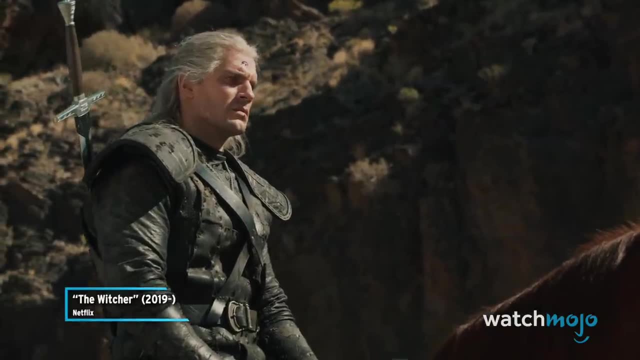 I'm gonna have to relieve you of your duties on this mission. That's disappointing. Number 13,: The Witcher. Netflix certainly tossed a coin to The Witcher. How is that song so catchy? Toss a coin to your Witcher. 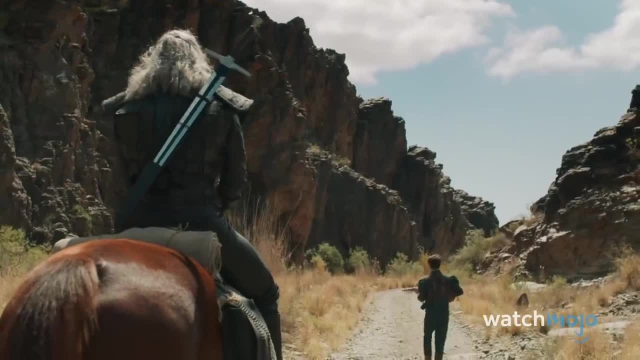 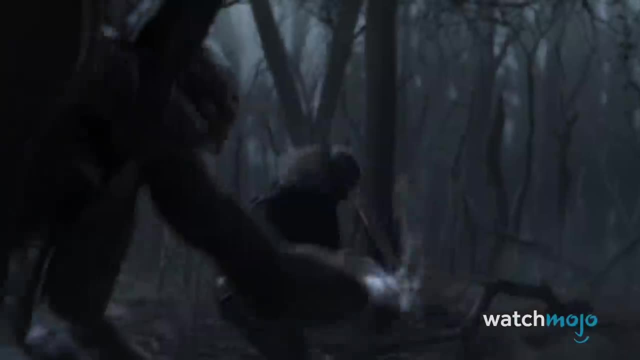 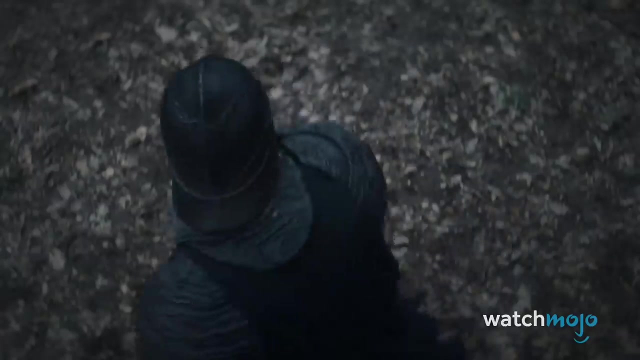 O valley of plenty. Besides infectious ditties, The Witcher also has plenty of epic battles, terrifying creatures, magic, as well as fantastic costumes, sets, actors and so forth to bring the world of the show and books and games to life. and books and games to life. According to reports, the whole first season cost between 70 and 80 million dollars to make, Which works out to around 10 million dollars an episode, And given that the series is only just beginning, that number is sure to increase down the line. 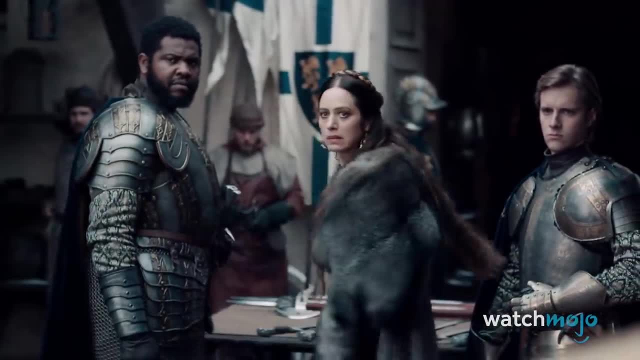 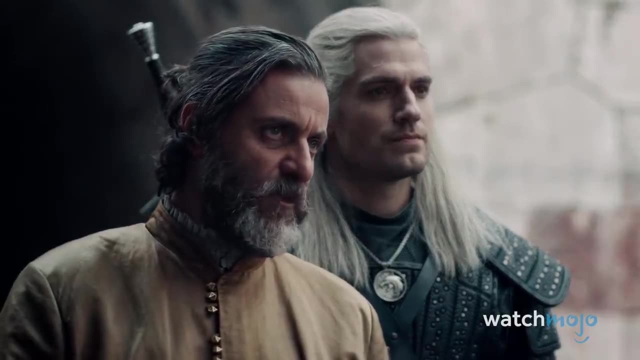 Move along Witcher Pay whatever you want. I can't be bought. Move along Witcher Pay whatever you want. You should remember money can't undo the law of surprise. number 12, Rome. I am a Roman citizen of noble birth and I order you to cut these ropes. 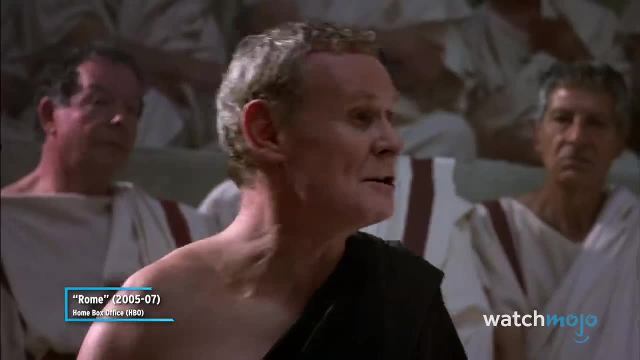 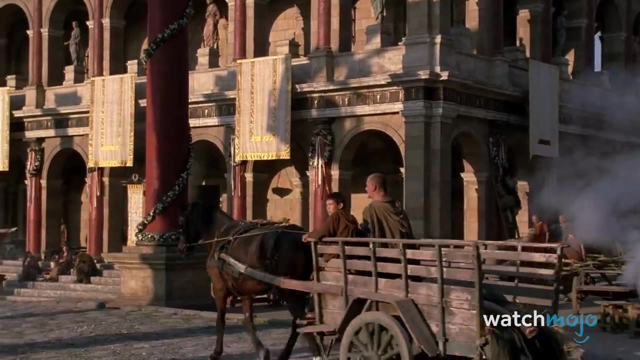 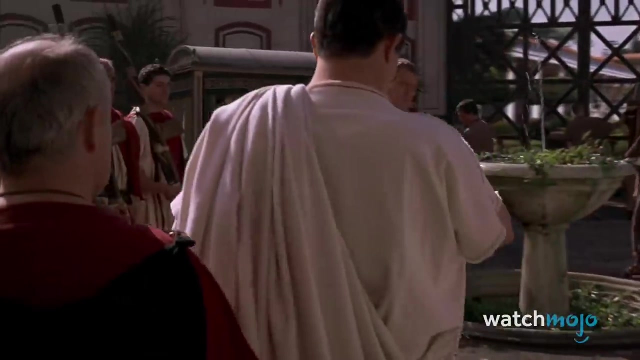 This was one of the first shows to prove that historical epics could work on the small screen as long as networks are willing to spend Accordingly. not only did the show feature a massive cast, it also required incredibly detailed set recreations of ancient Roman locations, Including Roman villas, slums and the forum. good day senator. 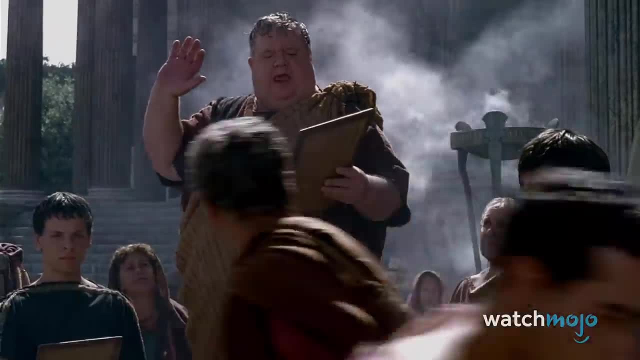 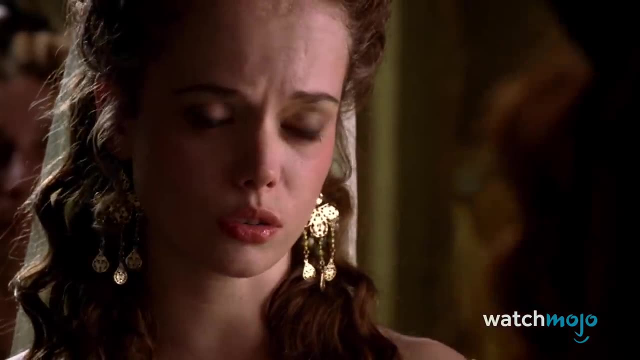 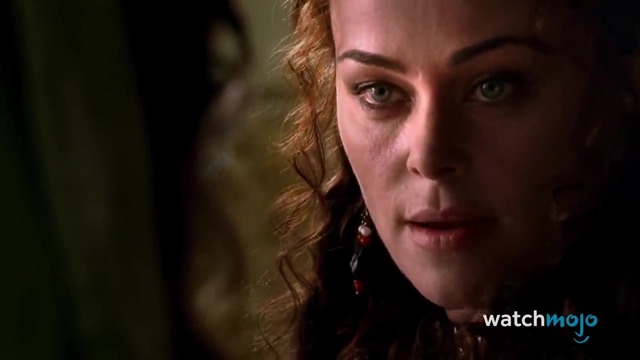 The daunting production costs resulted in HBO and the BBC splitting the budget of the show, which ended up costing nine million dollars an episode. Rome was a pioneer in putting epic stories on television, something that HBO would go on to explore with future shows. You're swearing now, someday. 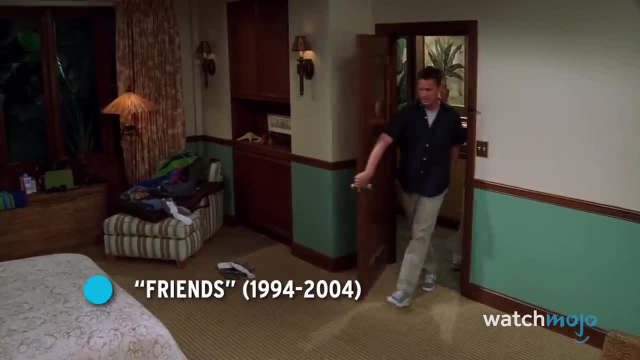 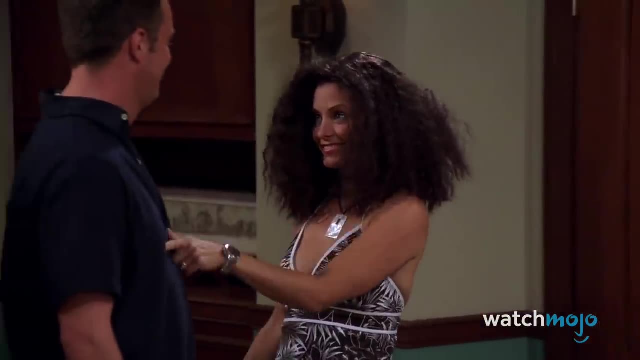 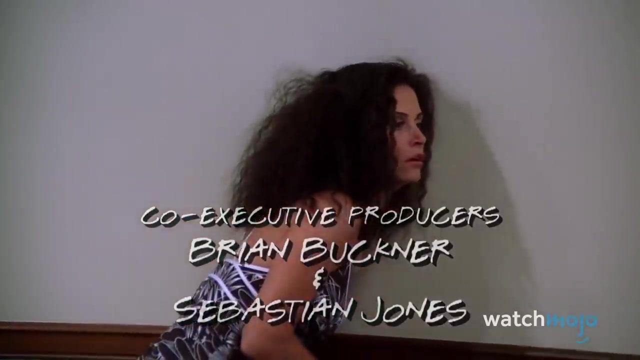 You'll destroy me. number 11 friends, the way You crushed Mike at ping-pong was such a turn on. You wanna big budgets aren't just the standard for sprawling prestige dramas. Sometimes, if a show has a talented enough cast, much of its cash winds up committed to keeping them around. This was the predicament NBC found themselves in with this must-see TV staple. As the six leads rose to popularity with the show, the cast maintained equal salaries, Which, towards the end of the series, was a substantial sum. for the final two seasons, Aniston, Cox, Kudrow, LeBlanc Perry and Schwimmer were all getting paid 1 million dollars per episode. 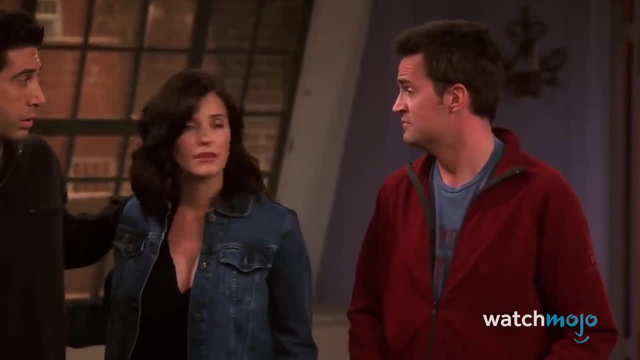 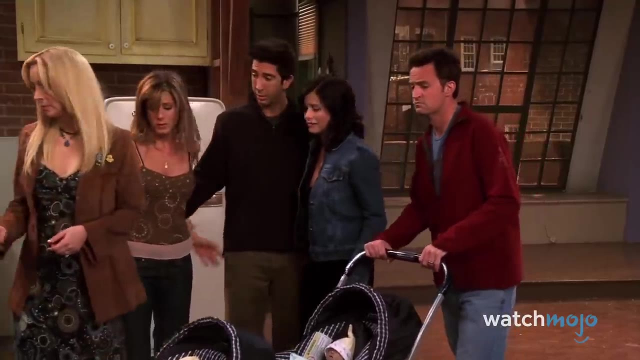 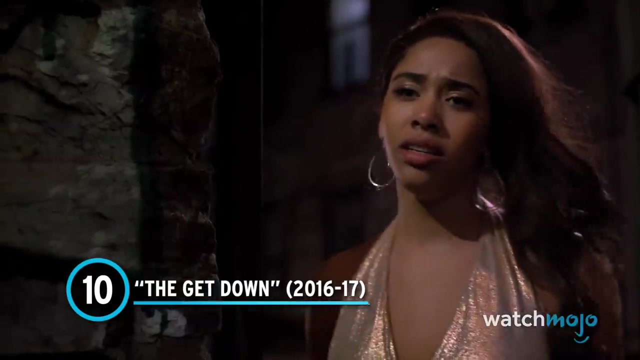 Jacking up the show's otherwise modest budget and making friends. one of the most expensive sitcoms ever produced. Okay, should we get some coffee? sure? Where number 10, the get-down? Molly, I know you like me. Thank you so much. I, Carly, breathe with a visual wonder, like Baz Luhrmann at the helm of the show. 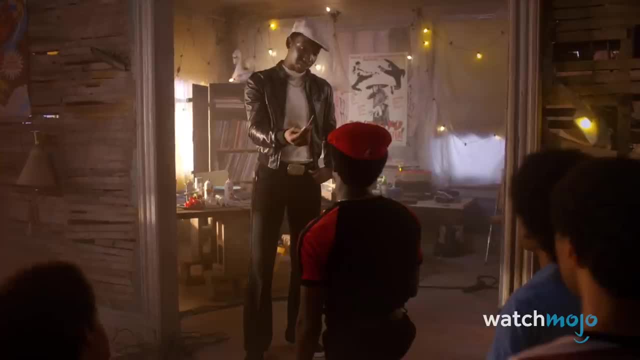 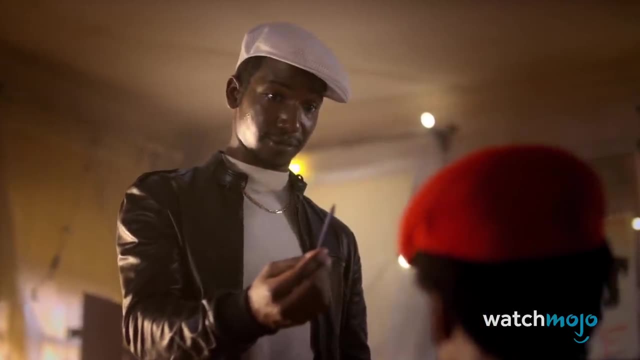 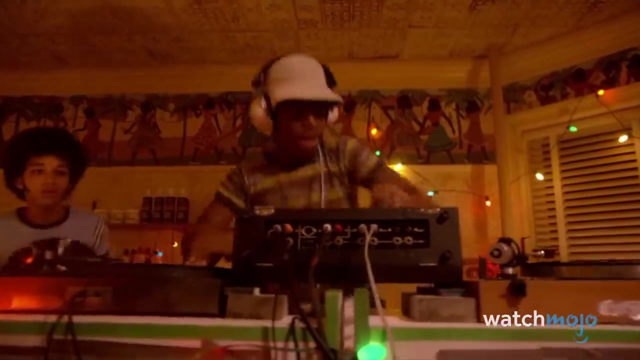 You know it's gonna be saddled with a Hollywood level budget. Indeed, his Netflix project is one of the most expensive shows ever made, especially for a streaming service. Put your hand on the position of Sun Tzu's offering. I hand you the magic: the show's recreation of 1970s New York. 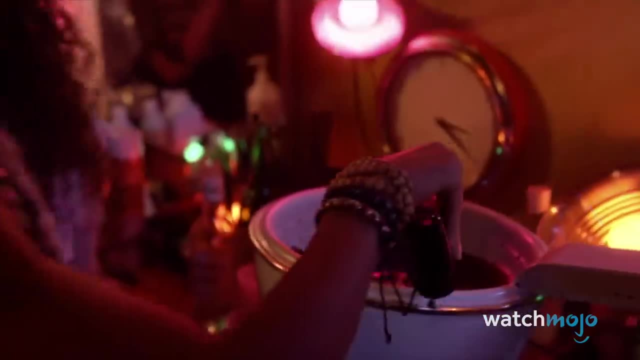 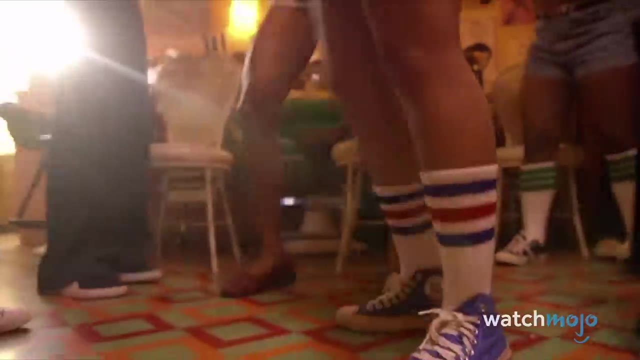 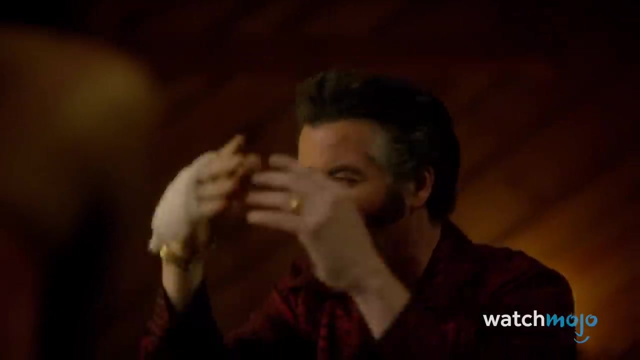 As well as lavish musical numbers, have given the show a price tag of 10 million dollars an episode, resulting in 120 million dollars for the 12 episode first season, Which is just 10 million less than Luhrmann's most expensive film, Australia. the world's dying of a thousand heart attacks. we 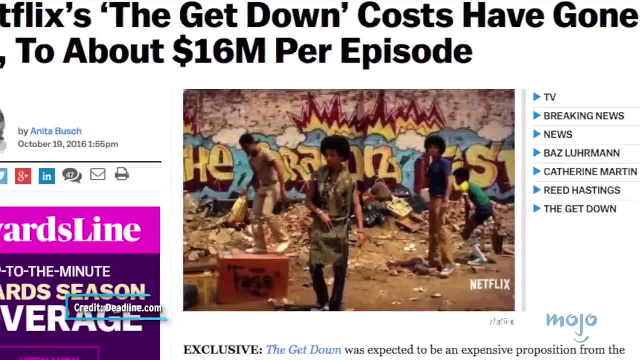 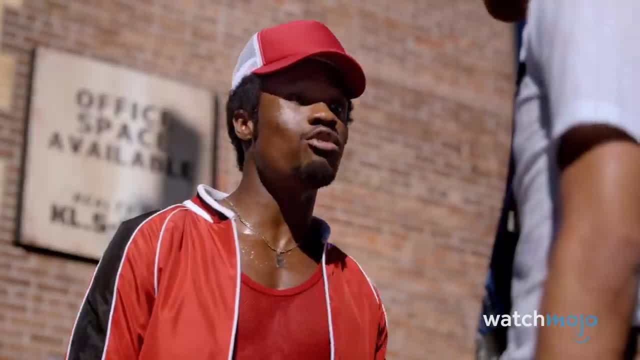 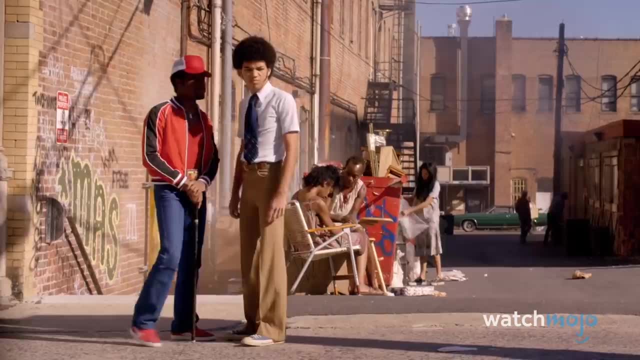 Heal them up three minutes at a time. although Unconfirmed, it's been rumored that it frequently went over budget, with sources claiming that it climbed to 16 million per episode, or roughly 192 million dollars total. so I'm B What? the first black Puerto Rican president. 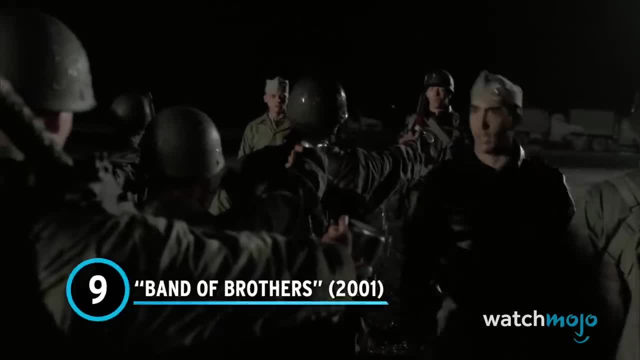 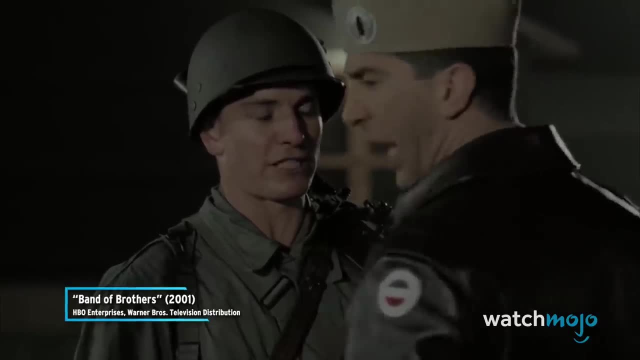 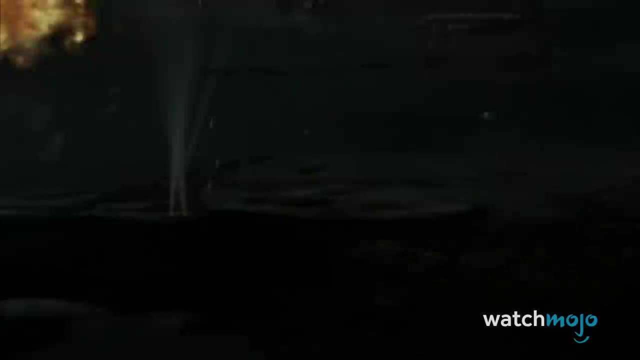 Yeah, what you trying to be, king number nine. band of brothers Christensen. Why is there no water in your canteen? you drank from your canteen, didn't you? a miniseries about a real company of soldiers who fought During World War two, band of brothers was the most expensive TV series ever created at the time of its release, and it certainly shows. 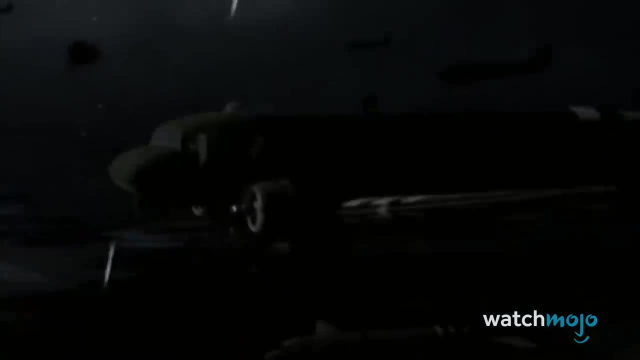 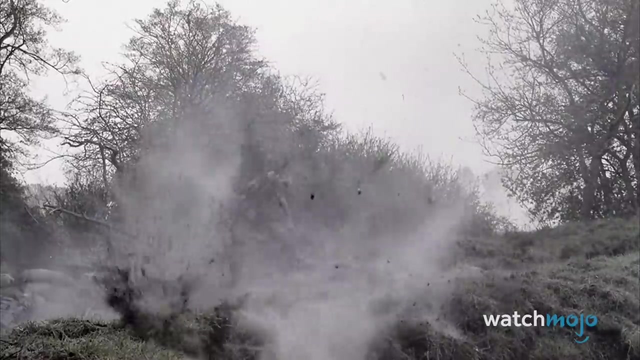 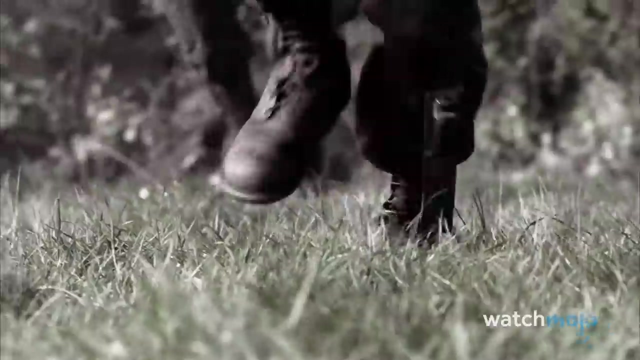 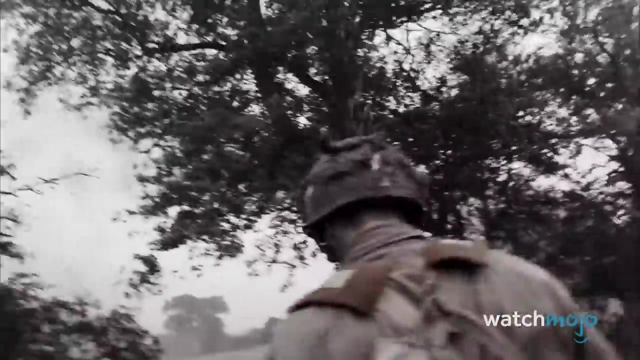 that it was made decades ago. Although it was made decades ago, the effects and battle sequences looked like they could have been shot today. They hold up that well, And a good thing, because the total cost to make the show was around 125 million dollars, which equates to twelve and a half million dollars for each of its ten episodes. 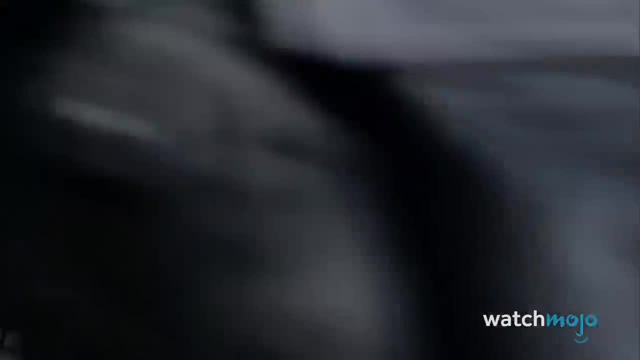 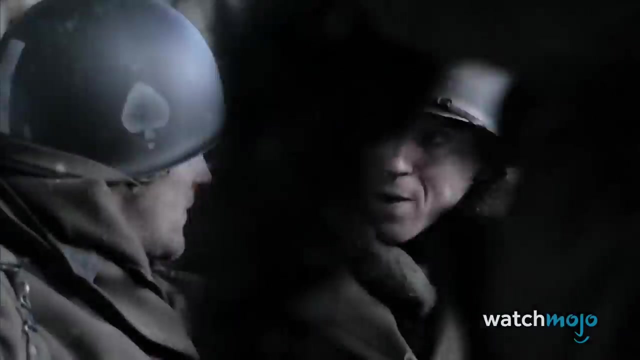 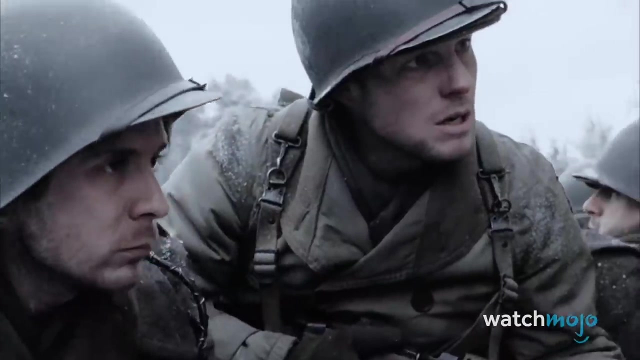 You got to move in there fast. Get in there before they can bring their mortars and artillery down on you. clear, Clear. I'm lying on you when it comes to telling the story of these brave men. However, no price is too high. You take your men on a flanking mission around the village. 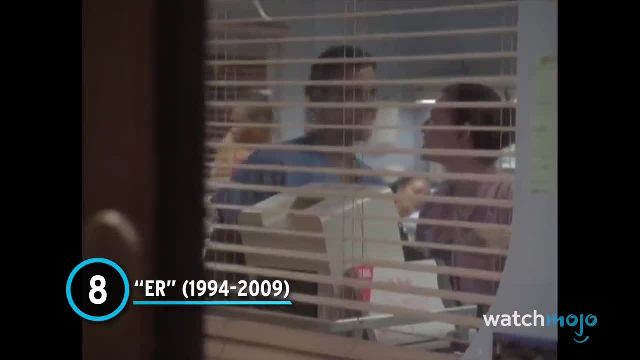 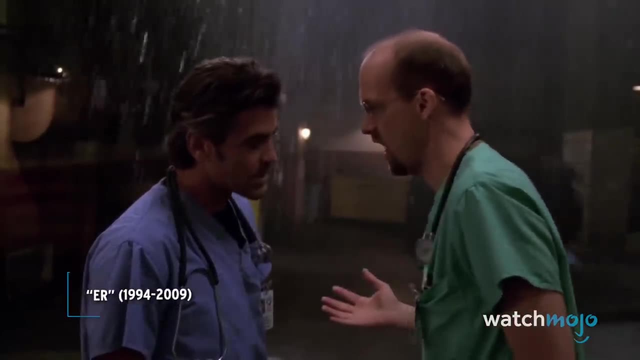 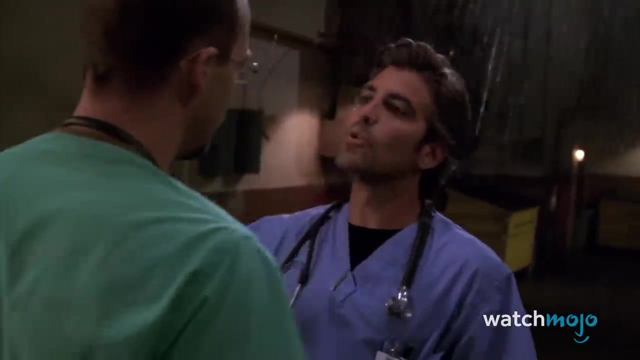 Number eight, er, a medical drama seems like an unlikely candidate for such a list, But then again, you series have held the title of most watched series in the country or included a young George Clooney. Like being disappointed in me. mark Validates the fact that you are the adult and I'm a screw-up in order to maintain high ratings and to keep their star player on board. 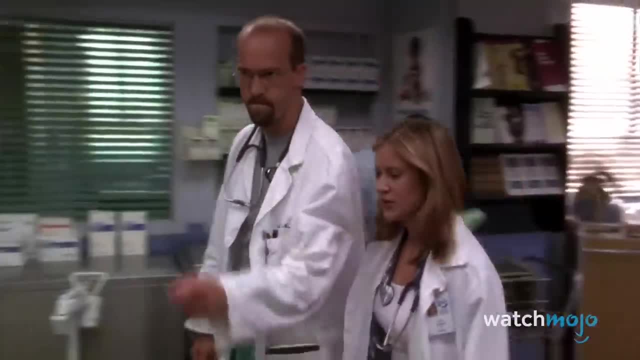 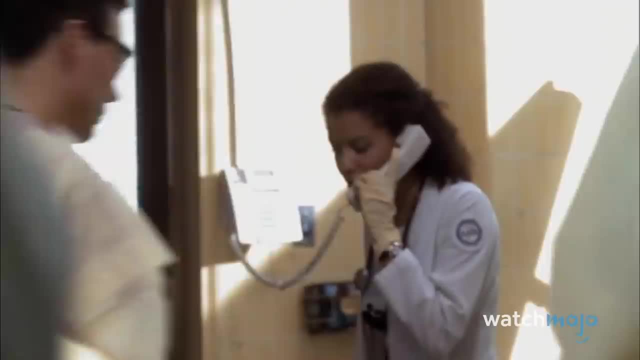 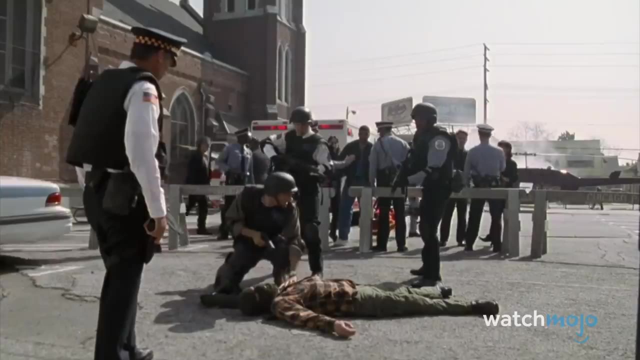 NBC bumped the per episode budget from two million dollars to a whopping 13 million for seasons four through six. The investment was later known by some as the half a billion dollar blunder, Costing NBC a whopping four hundred and forty million dollars. All right, Squeezing that own egg as fast as you can. still, er stayed in the top five in ratings during that time. 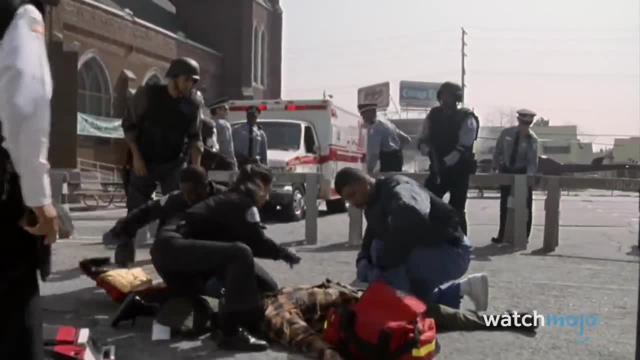 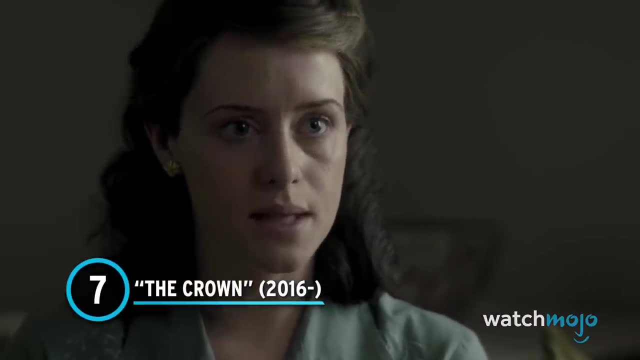 Though Clooney checked out at the end of the fifth. sir, I'm a doctor, I'm here to help you. Can you talk? Okay, I'll take that as a yes. number seven: the crown. My name is Elizabeth. Long live Queen Elizabeth. It's only fitting that a show about the royal family ends up being jaw-droppingly expensive. Another Netflix period drama, the crown, had a budget estimated to be in the ballpark of one hundred and thirty million dollars Just for the first season of ten episodes, if accurate. 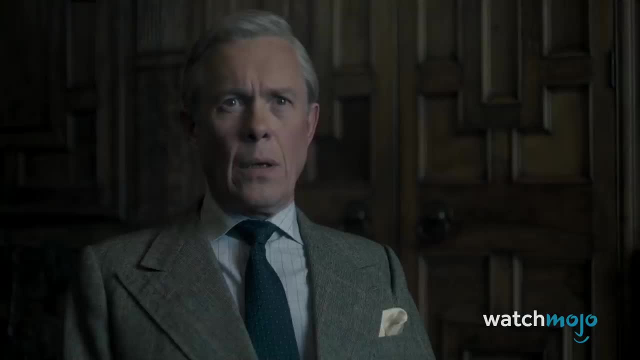 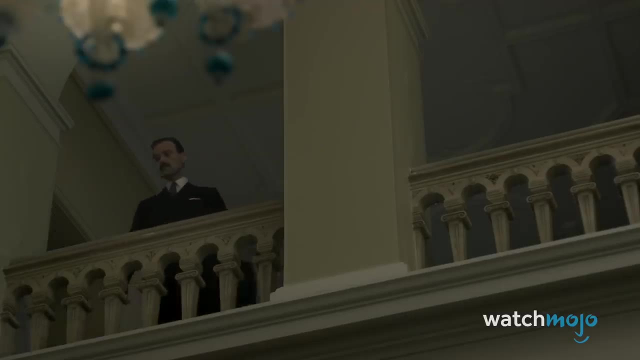 Then it's quite obvious why this show makes our list of the most expensive TV shows in history. Oh, it's mad. Once again, the massive budget comes as a result of incredible period detail, Which includes such things as a realistic recreation of Buckingham Palace and roughly twenty thousand costumes. 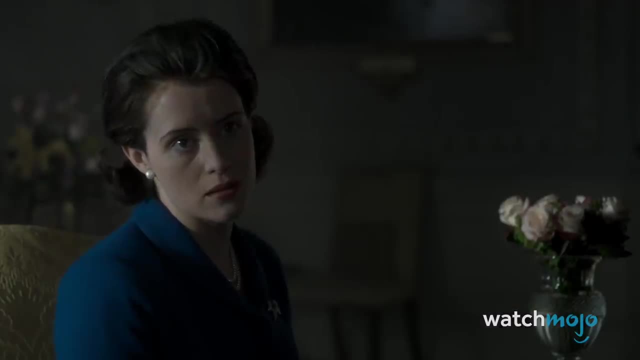 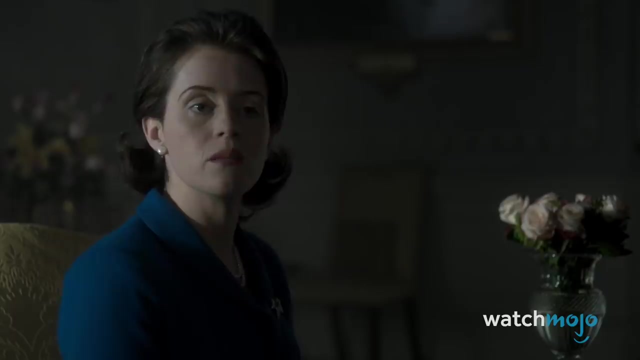 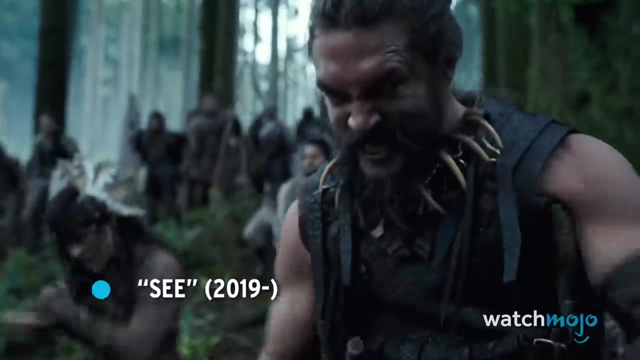 Lucky for Netflix, the gamble paid off, as the show has received strong reviews and viewership. It's a noose that we both made and that We intend to keep. number six: see. See is set in a post-apocalyptic world where most humans have lost the ability to well see. 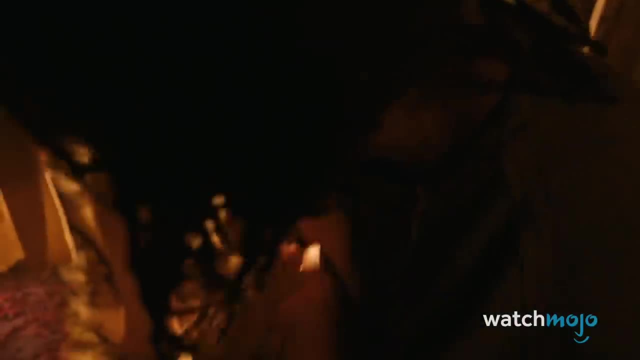 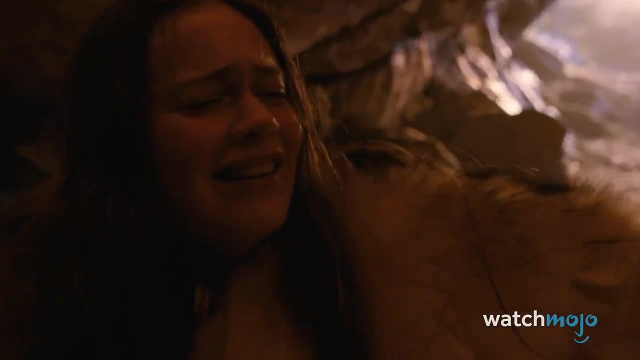 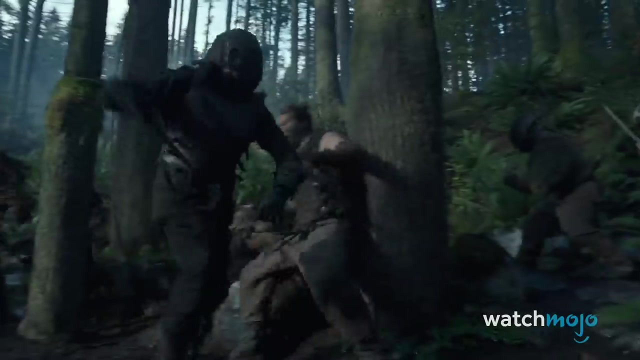 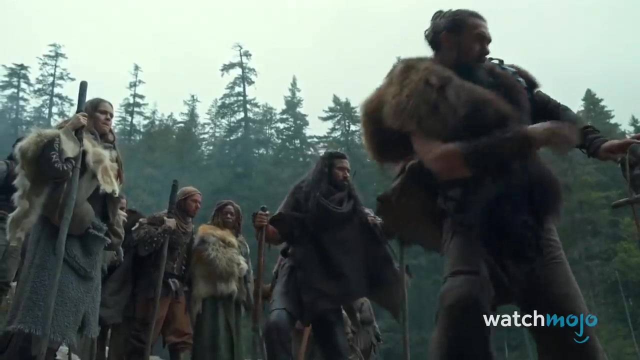 It follows a tribe in the mountains that comes under threat when two children are born with sight. Apple TV plus has allegedly spent a cumulative 240 million dollars on the first and second season, which works out to around fifteen million dollars per episode. While the show has received some mixed reception thus far, the streaming service isn't just throwing their money away. I will go first. 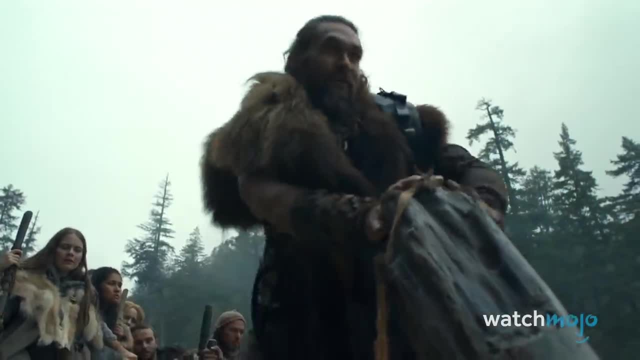 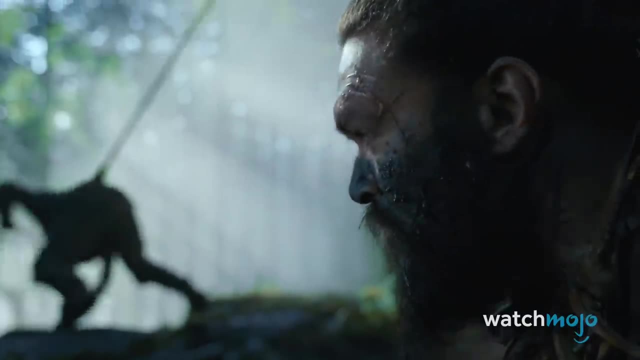 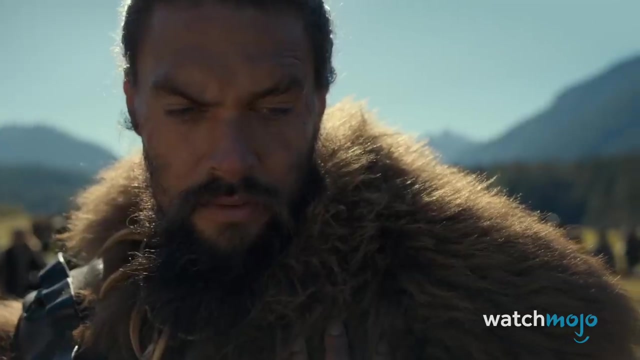 You can hold my weight. You can hold anything, Please see, has impressive effects, epic Battle scenes and some big star power. with actors like Jason Momoa and Alfre Woodard, You will be chief of a tribe That must hide from the world and the witch finders forever. number five, the morning show. 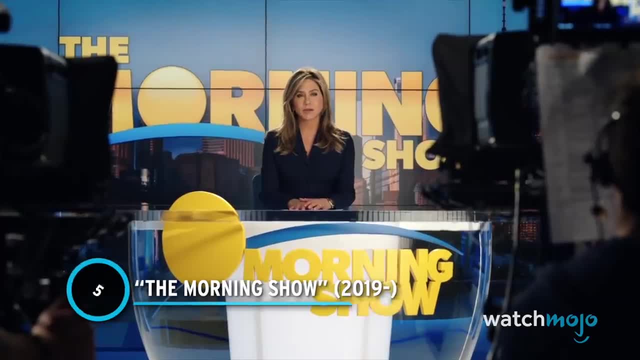 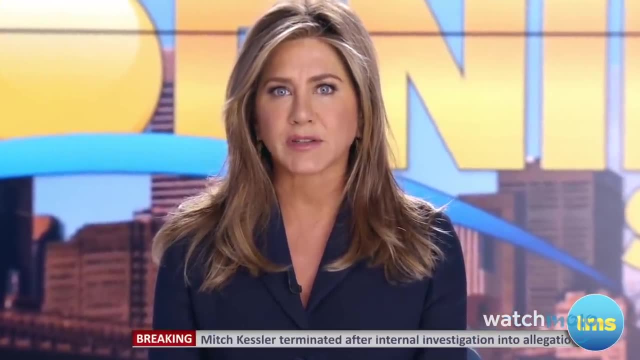 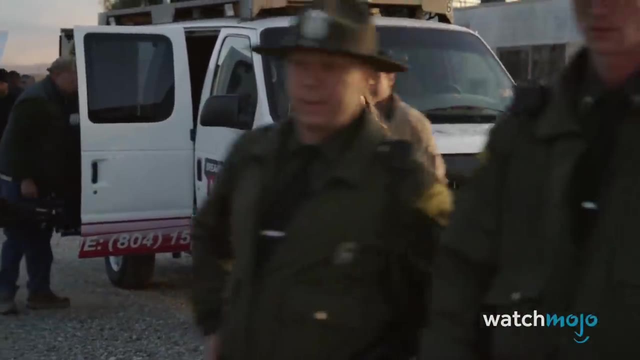 Speaking of the Apple streaming service, one of its other big offerings is the morning show. Mitch Kessler, my co-host and partner of 15 years, was fired today for sexual misconduct. a dramatic look into the competitive world of Morning news shows. the series highlights a toxic culture that feels ripped from the headlines and 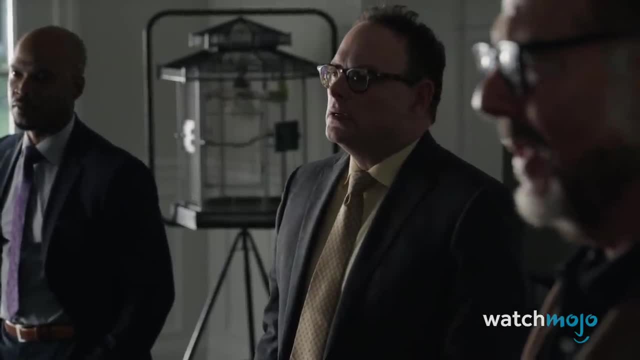 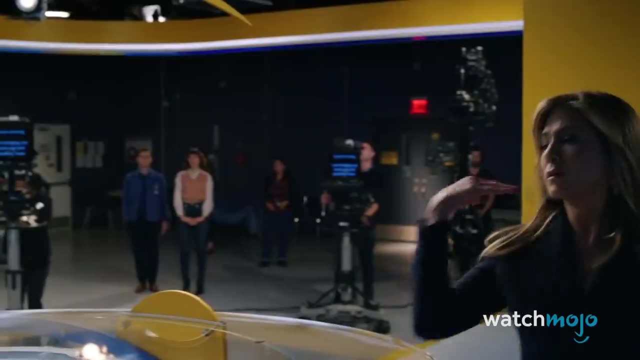 Certainly real-world morning news shows. the network that I gave 20 years of my life plus is now locking me out, Throwing me the wolves. They won't even engage in the discussion with me. It has been widely reported that the morning show has a budget of around 15 million dollars per episode. 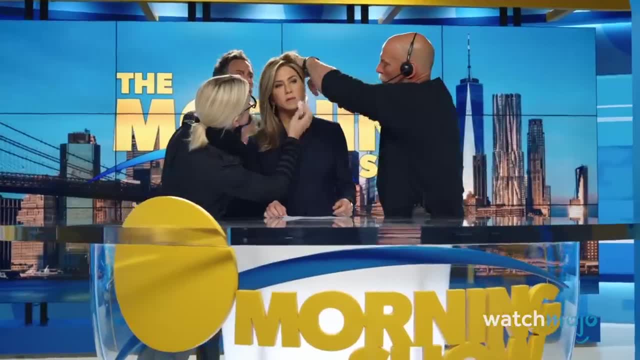 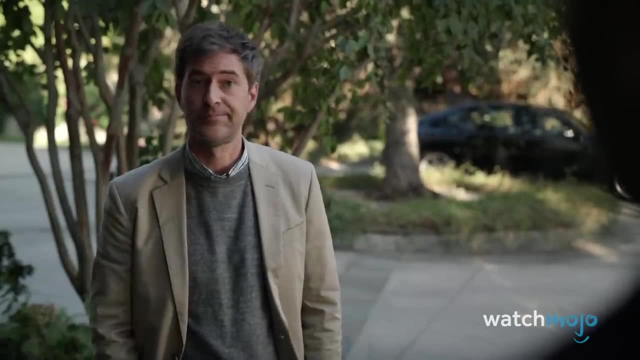 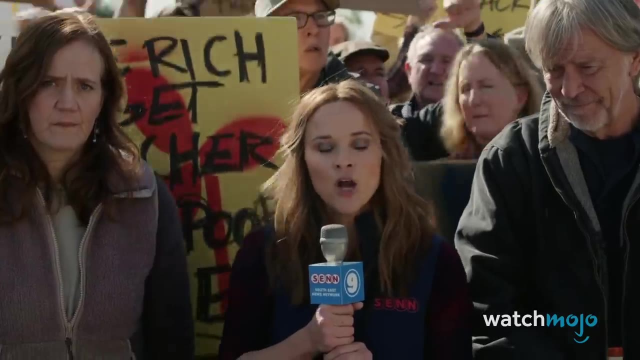 Although some who have worked on the show dispute this number, calling it inflated. How long do I have to sit around while I take my punishment like a man? I Don't know. I don't know what the half-life is on this, But I know it's not a day still, with stars like Jennifer Aniston and Reese Witherspoon making two million bucks an episode. 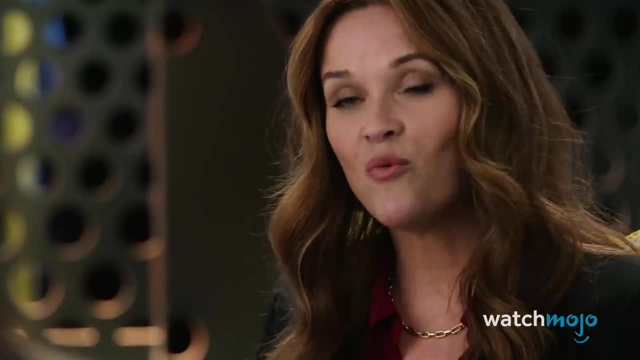 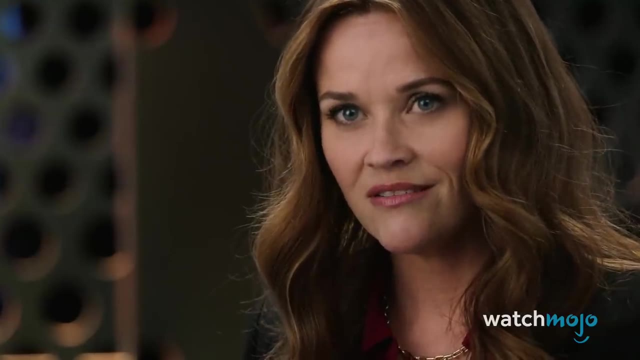 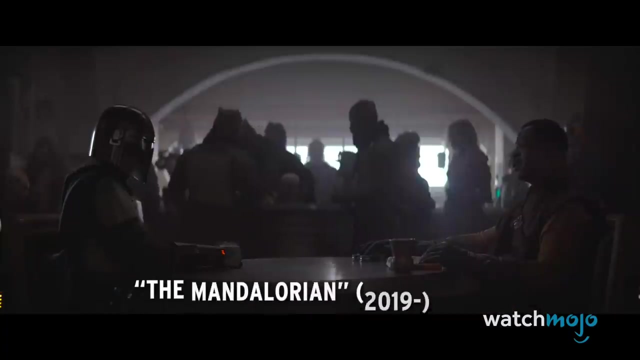 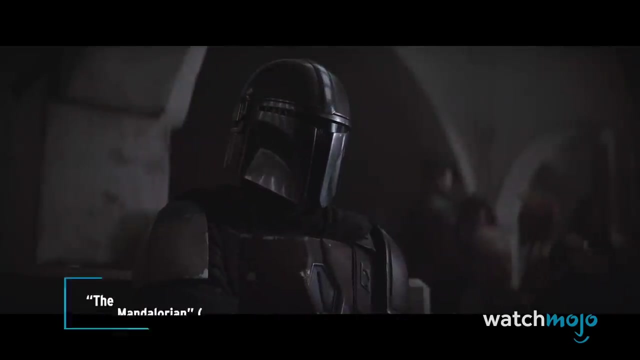 Those estimates do not seem unreasonable. I think they want to trust that the person that is telling them the truth about the world is an honest person Like you. number four, the Mandalorian Star Wars is big business, but it also costs a lot of credits. What's your highest bounty? not much. 5,000, they won't even cover fuel these days. the hit Disney plus show about a lone bounty hunters adventures in the Star Wars galaxy Looks just like the movies. The numerous creatures, costumes and effects are all top-notch and wouldn't look out of place on the big screen. 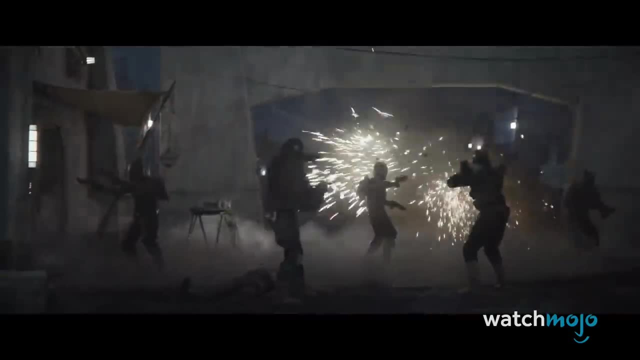 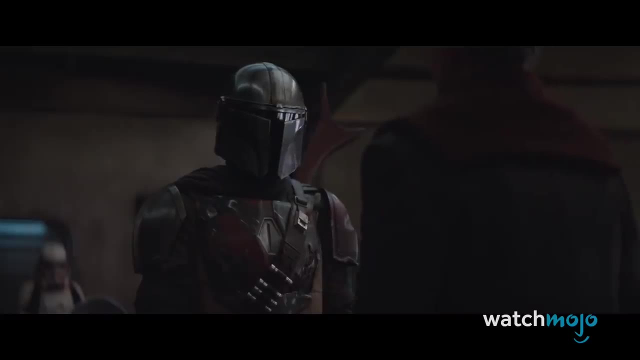 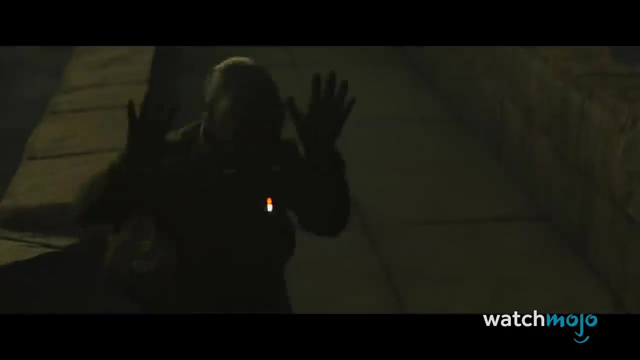 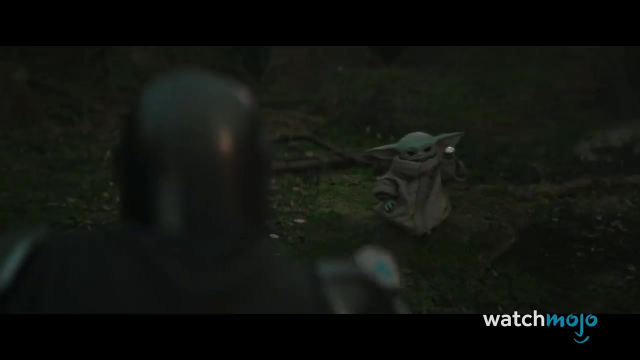 And we sure hope so. given that it reportedly cost about 15 million dollars an episode, you have taken both commission and payment. Is it not the code of the guild That these events are now forgotten? still, given how successful the show has been, Disney has no doubt recouped that investment. and then some, the baby Yoda, merch alone must have made them a pretty penny. 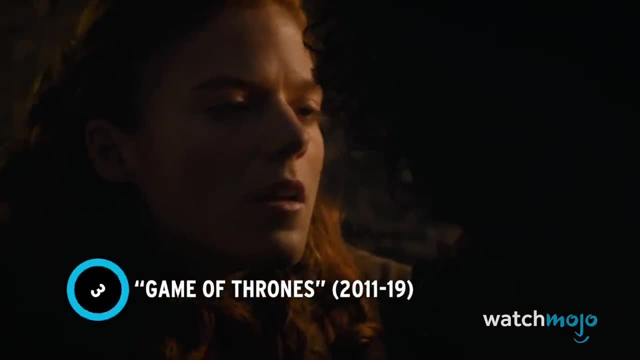 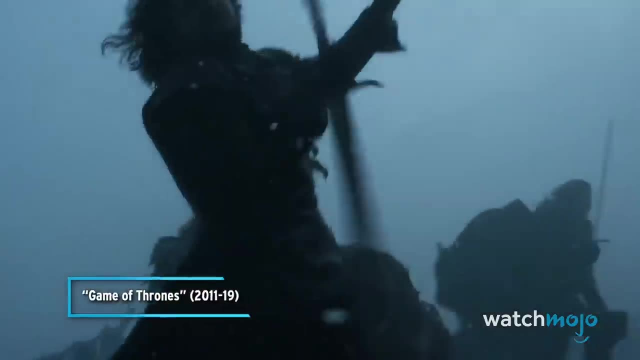 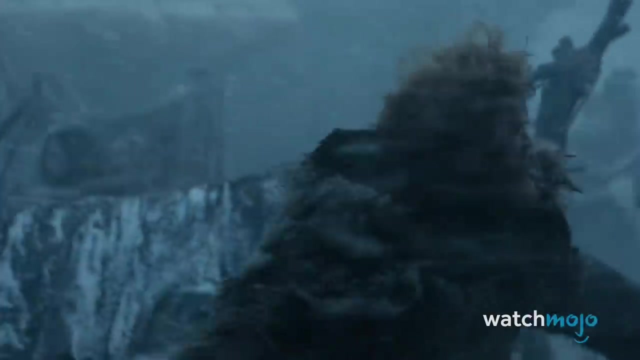 Good job, Good job, kid. number three, Game of Thrones. You know nothing. Other shows may have cost more, But there's no show on television that got a better bang for its buck than HBO's epic fantasy drama. in season one. It may do with a total estimated budget of between 50 and 60 million dollars. 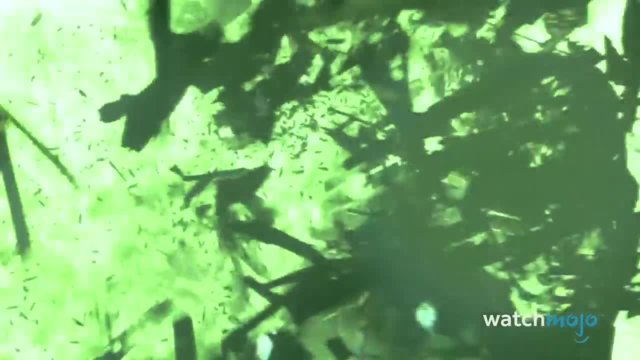 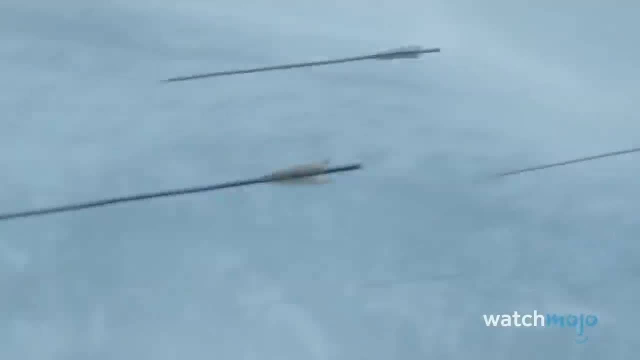 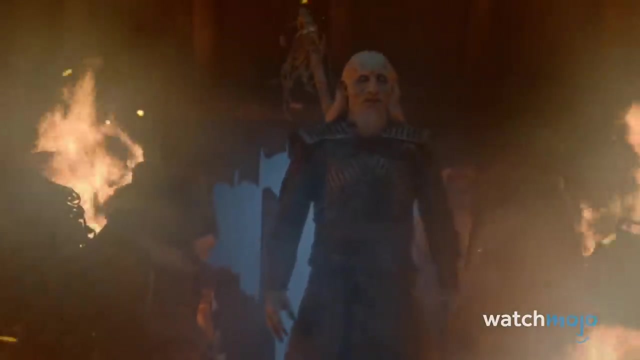 But after receiving a budget increase for season twos epic battle episode Blackwater, the price tag for the show steadily grew. By its final season, it was at 15 million dollars In episode. The high costs are put to good use, though, as the show features incredible effects for elements like the white walkers. 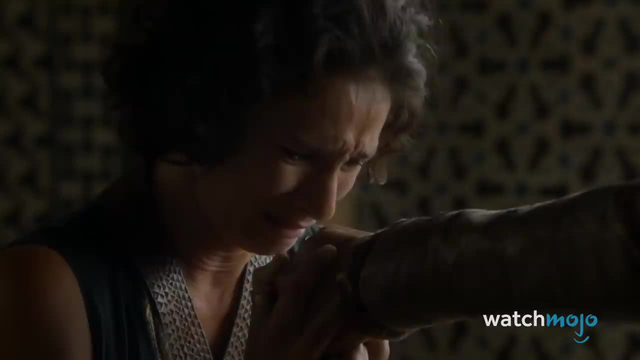 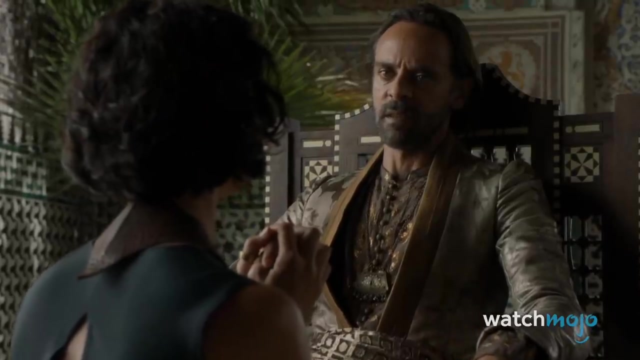 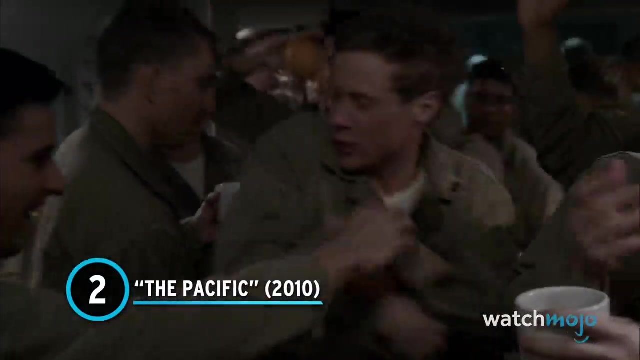 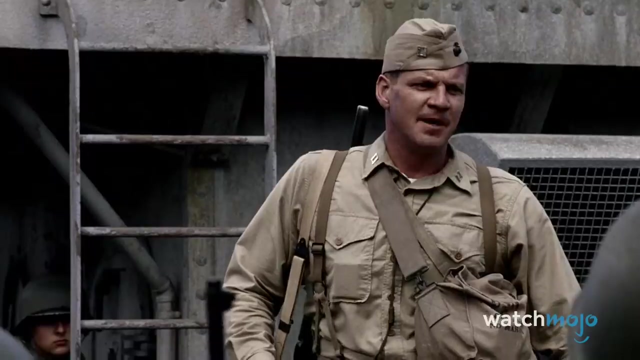 Dragons and huge battle scenes, as well as a stellar cast. Nobody, even second chances. And what even third chances. number two: the Pacific. Often seen as a companion piece to Band of Brothers, the Pacific focuses on the Pacific theater of World War two. The treacherous bastards may have started this war, but I promise you we will finish it. 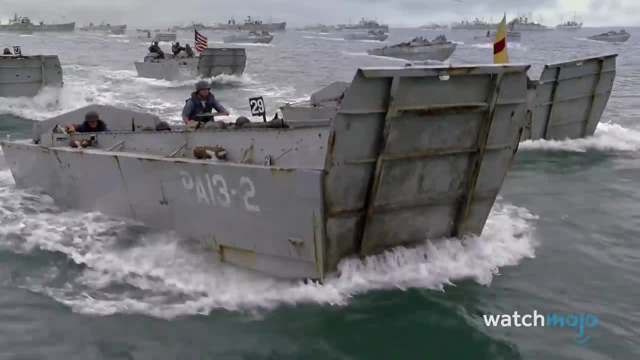 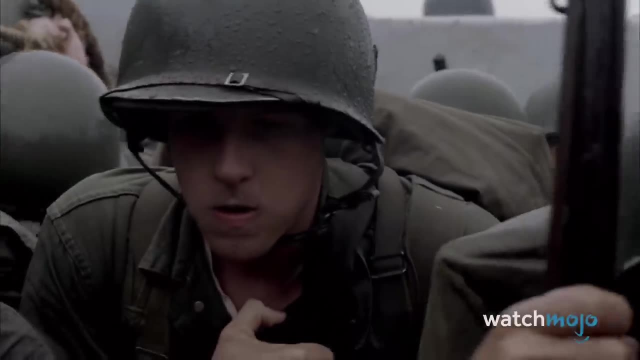 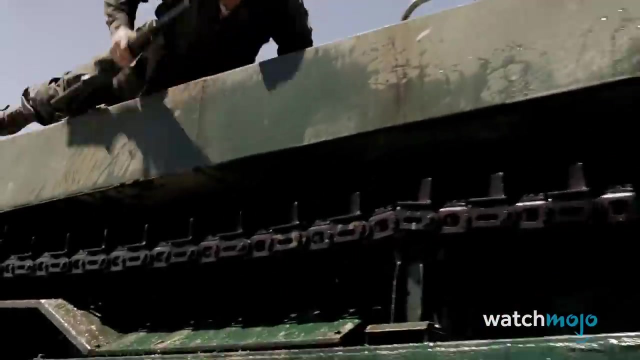 Yeah, However, it has nearly twice the budget per episode of the former series, costing around 20 million dollars apiece, for a grand total of 200 million dollars. some estimates actually place it as high as two hundred and seventy million. Here we go, Let's go, Let's go, Move, Move, Move. 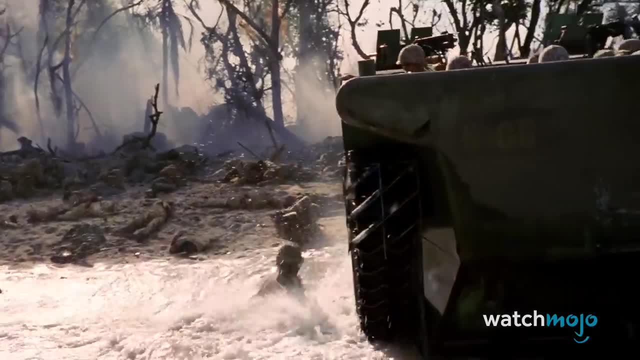 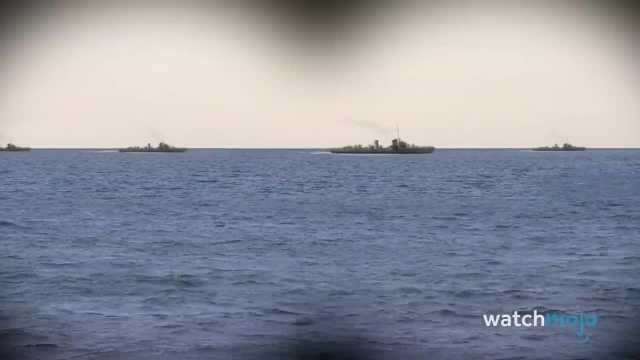 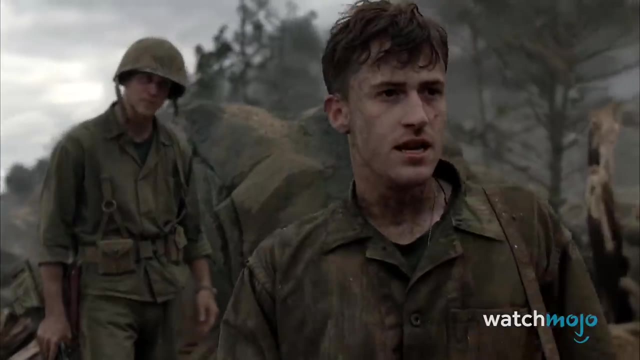 Go, Go Go. Given how epic, gruesome and realistic the battle scenes are, with many using practical effects, It's easy to see where all that money went. as of this writing, The Pacific is the most expensive TV show ever made. Just gave away our goddamn position. 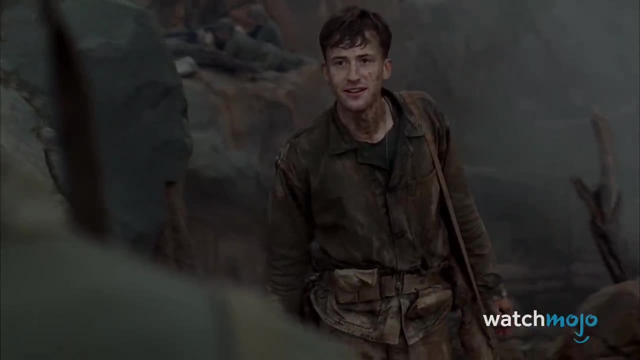 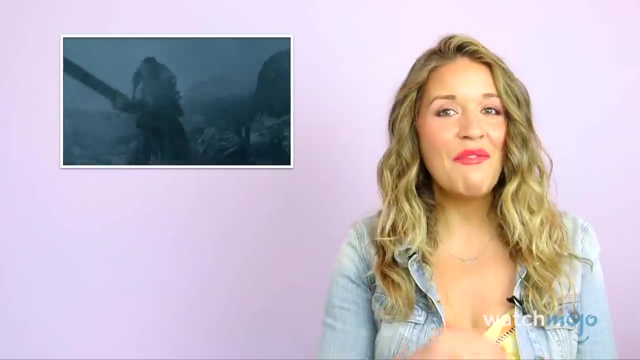 I think they got a pretty good idea of where we are. I told you to cease fire. Are you supposed to be observing? So why isn't it our number one pick? You'll find out soon. I find it funny that some shows are expensive because of sets and travel and CGI and action set pieces and that kind of thing and 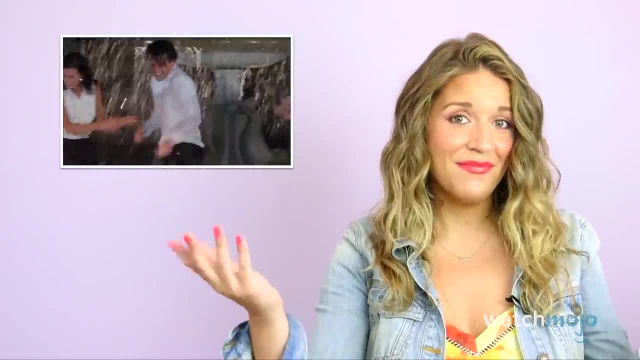 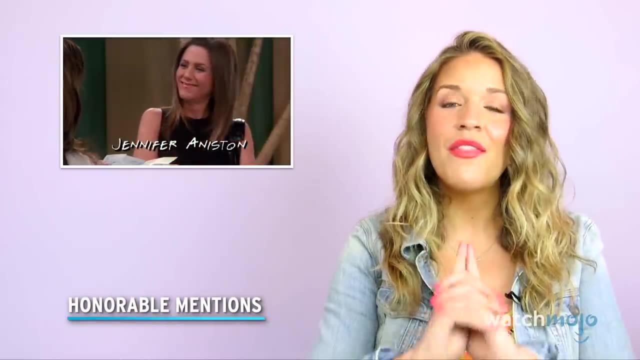 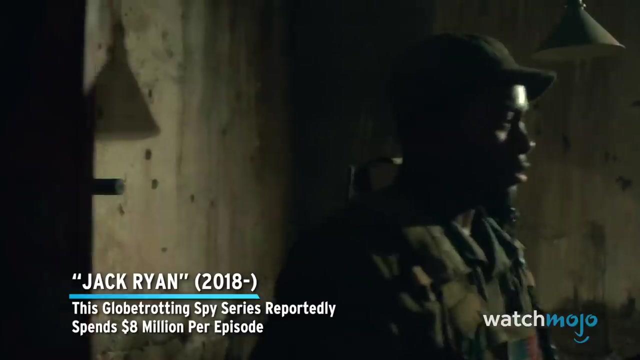 Some are expensive because their cast is mainly A-listers. Anyway, which category does our number one pick fall into? Let's look through some honorable mentions and then we will name the most expensive TV show ever made- Jack Ryan. this globetrotting spy series reportedly spends eight million dollars per episode. 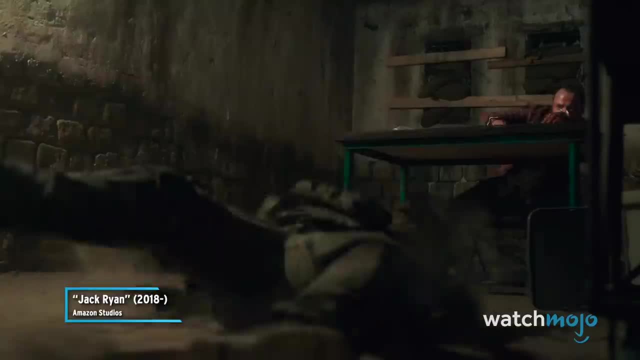 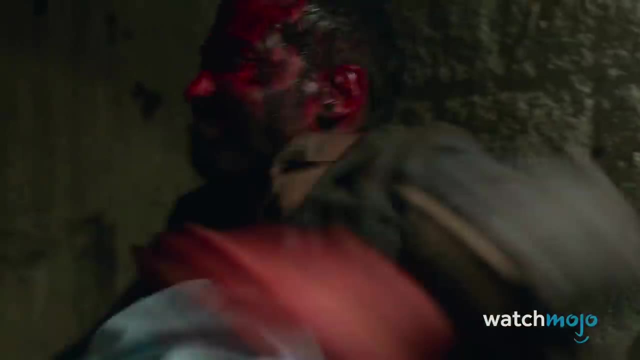 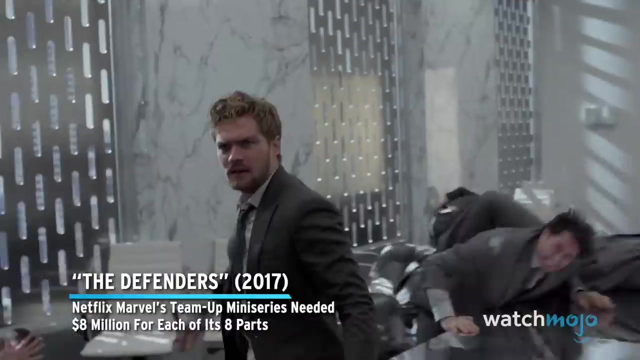 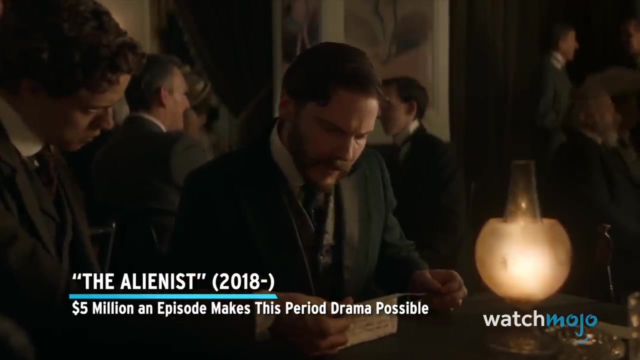 You bet what I bet One: The Defenders. Netflix Marvel's team-up miniseries needed eight million dollars for each of its eight parts, so punching's okay. now The Alienist. five million dollars an episode makes this period drama possible. I want to inflict pain. 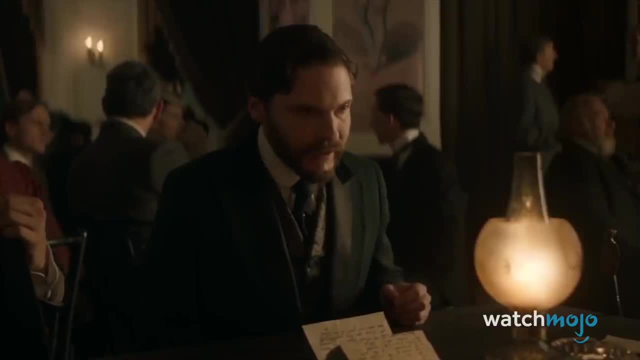 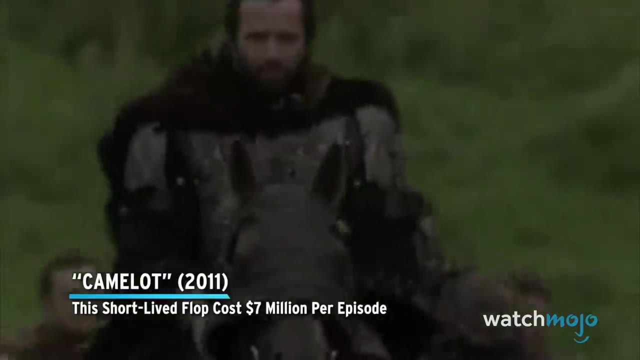 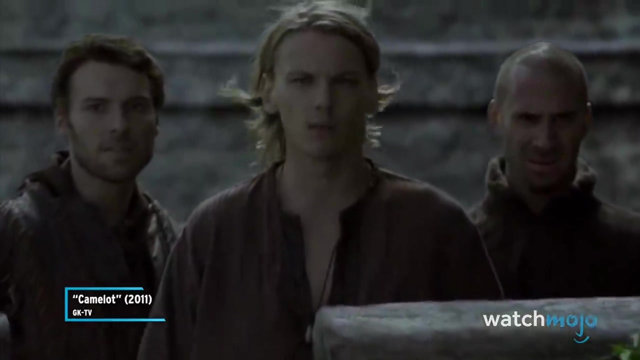 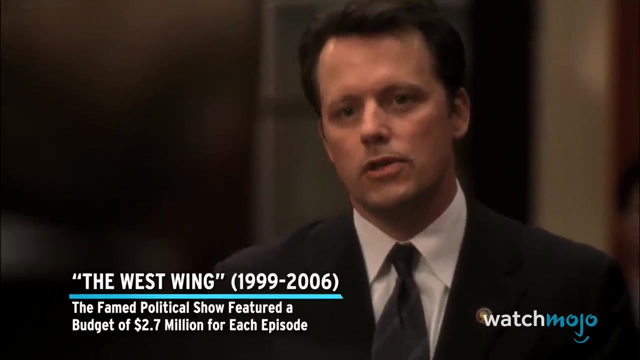 I won't be satisfied unless I can see the suffering that I'm causing. He was watching the Santorellis Camelot. this short-lived flop cost seven million dollars per episode. God help me. What do we do now? The West Wing, the famed political show, featured a budget of 2.7 million dollars for each episode. 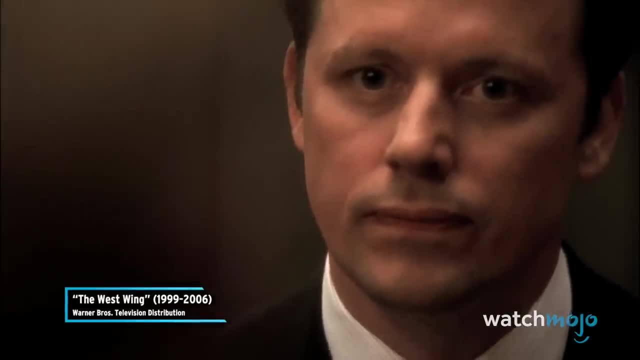 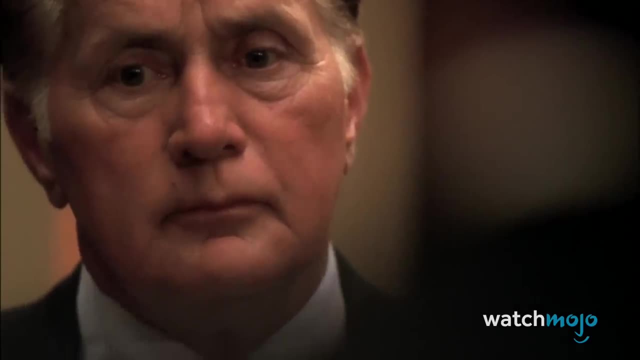 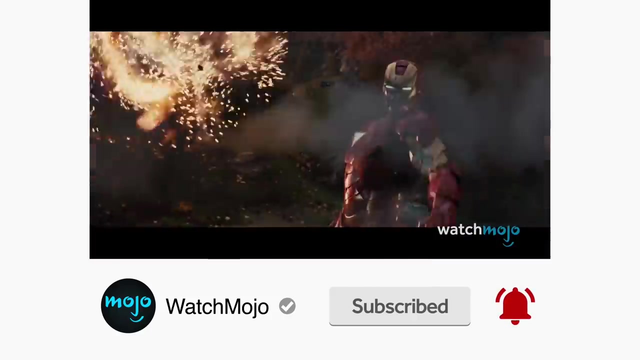 We will not vote to keep on footing the bill. You will be held responsible for shutting down the federal government. Before we continue, be sure to subscribe to our channel and ring the bell to get notified about our latest videos. You have the option to be notified for occasional videos or all of them. 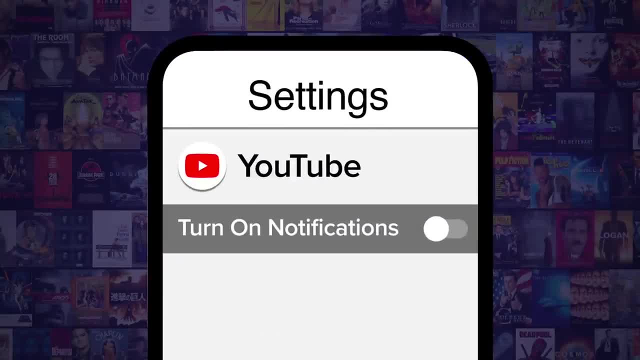 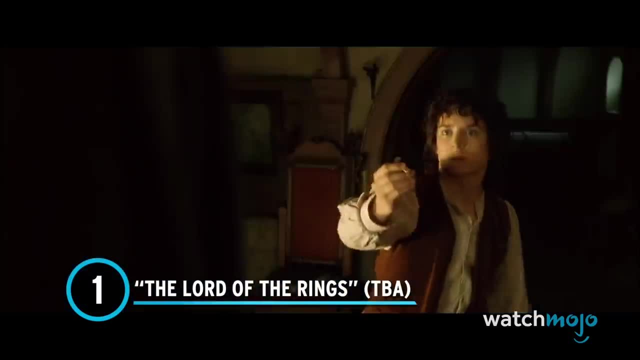 If you're on your phone, make sure you go into your settings and switch on notifications. Number one: the Lord of the Rings. The Lord of the Rings is one of the biggest names In fantasy and pop culture. you must take it. You cannot offer me this ring. I'm giving it to you, Don't. 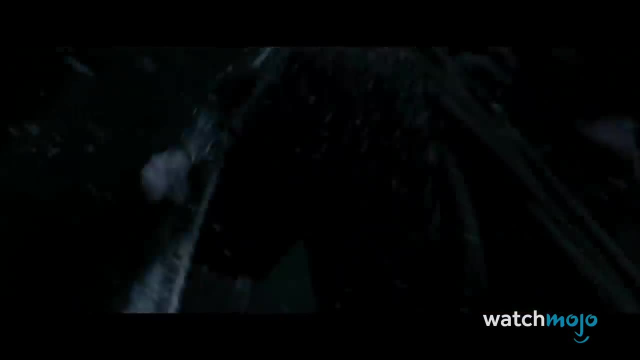 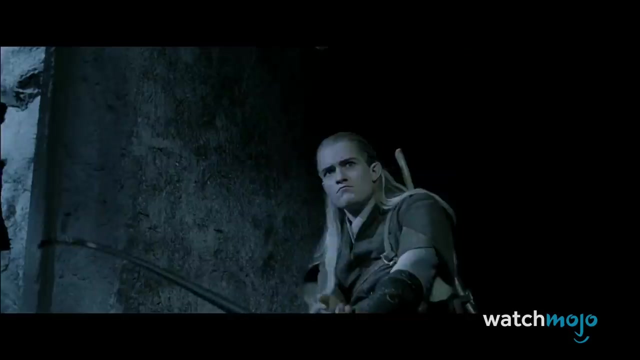 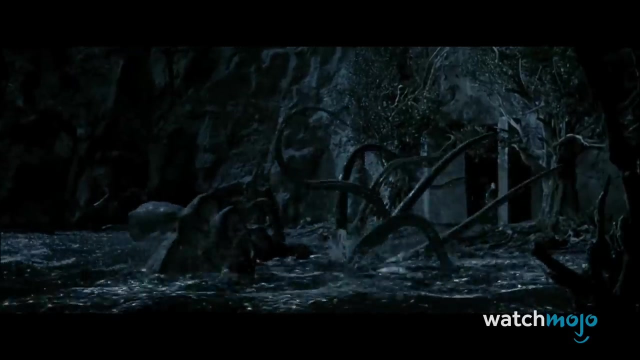 catch me photo. Amazon's forthcoming prequel, adaptation, is supposed to be set thousands of years before the books and films, though precious little is known about the plot yet, MrKnight. What is known, however, is that Amazon has spent two hundred and fifty million on the rights alone. 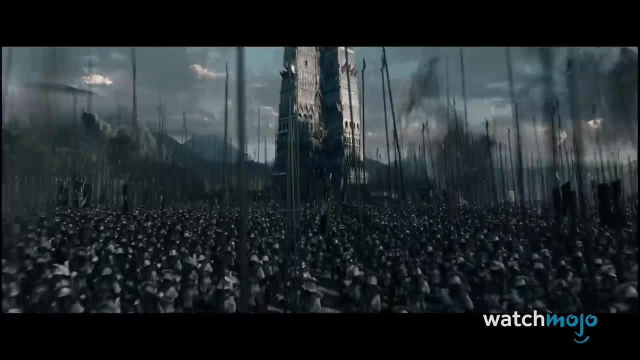 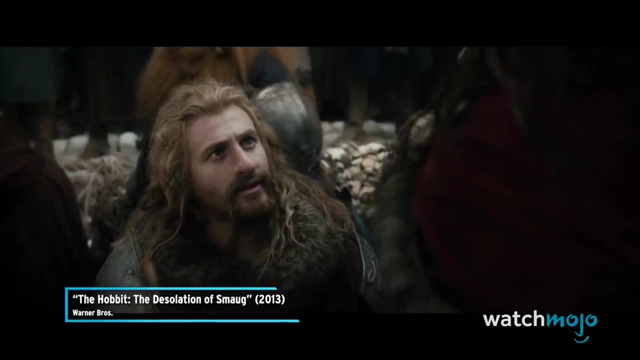 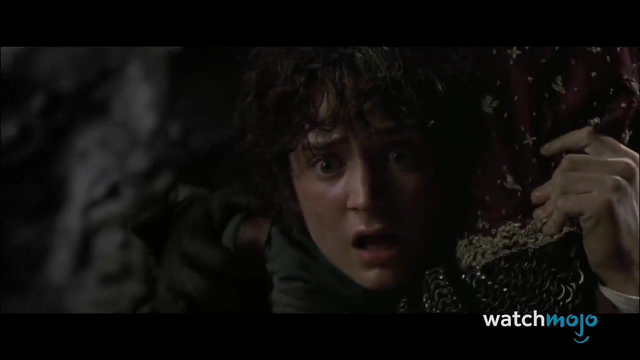 Not only that, but the estimated budget for each of the planned five seasons is set to be between 100 to 150 million dollars each. This would put the total amount spent on the series somewhere in the neighborhood of a billion dollars. That's dragon horde money or pocket change for Amazon CEO Jeff Bezos. 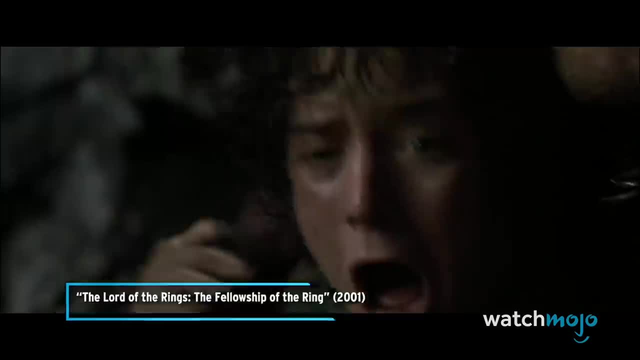 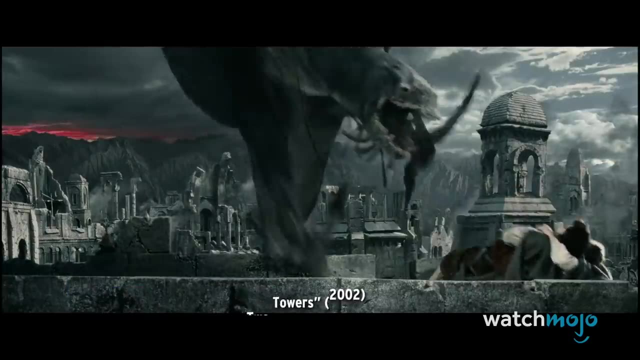 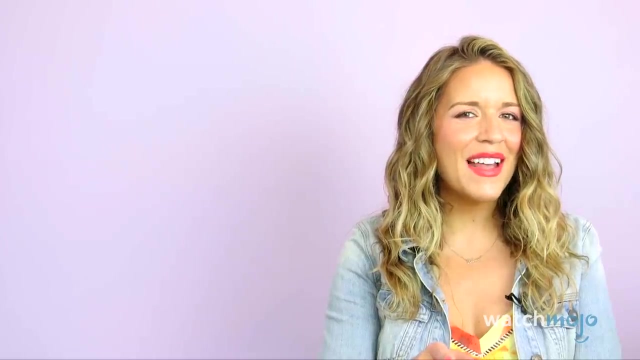 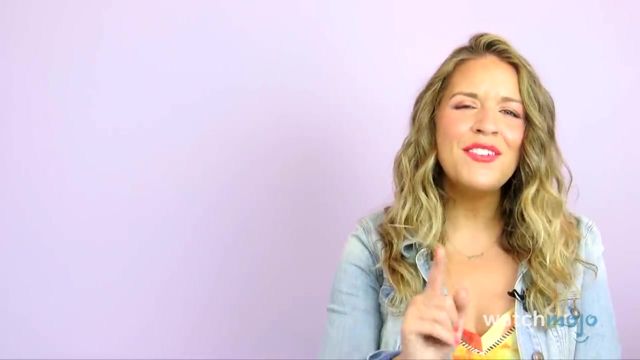 NOOOOOOOOOOOOO, We cannot wait to see the results. I'm pretty sure we covered this category on our game show What the Lisp, which is available now on our YouTube channel, Game Show Mojo, by the way. But anyway, do you think it's worth it to spend more money on a show? 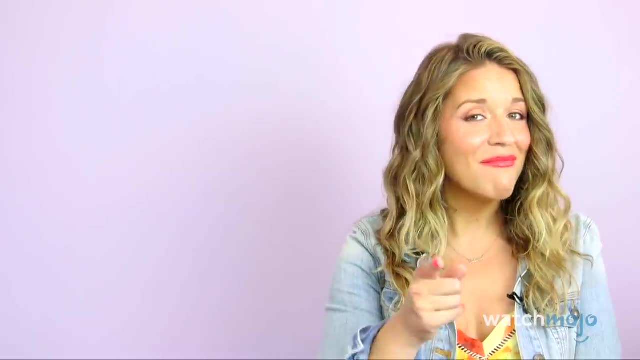 And also, are you excited for the Lord of the Rings show? Be sure to let us know in the comments, or come talk to me on Twitter or Instagram or on my YouTube channel. See ya. 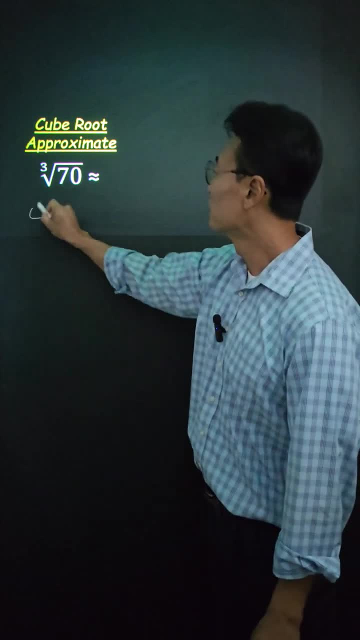 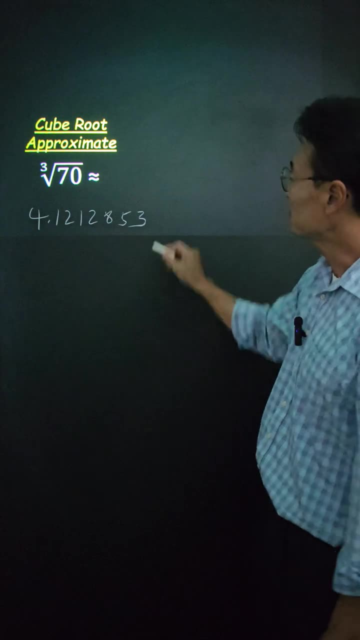 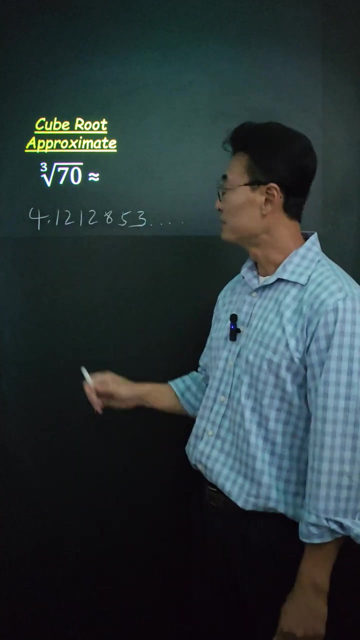 If you put cube root of 70 in the calculator, it'll give you 4.1212853, but since that's an irrational number, it means it goes on forever. Your calculator just doesn't show you the rest. To approximate cube root of 70, here's what you do: First take the cube root of 64, because that's. 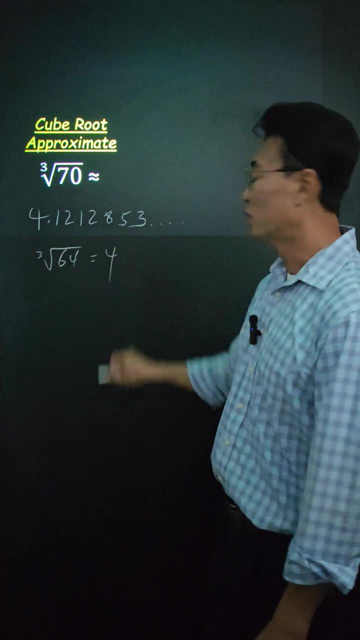 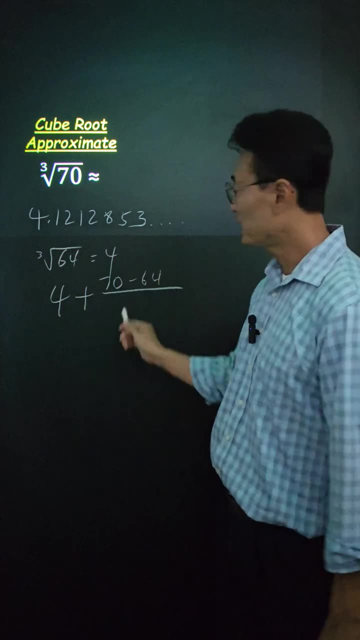 the biggest perfect cube less than 70,, which is 4.. Then you take the 4, add the difference of 70 into 64, divide it by 3 times 4. squared, The 3 is always going to be 3 because we're taking the. 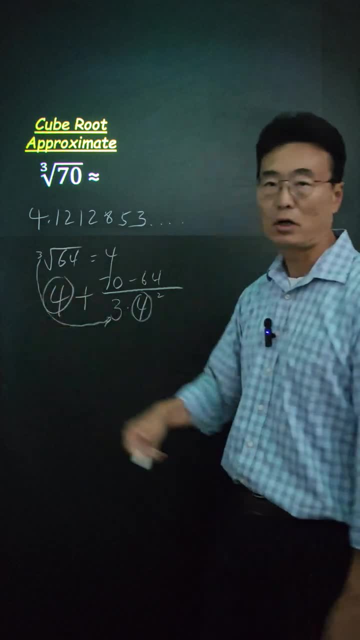 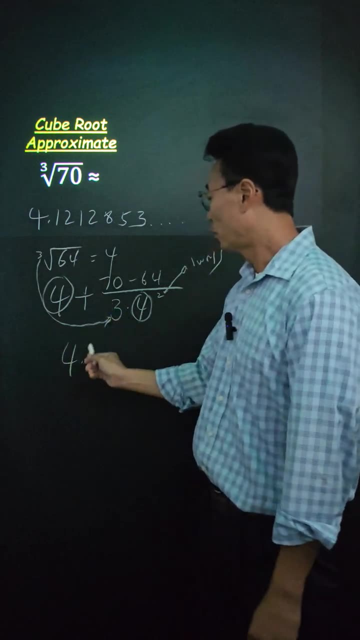 cube root of The 4 here and the 4 here will always match up, and then 2 is always 2.. Then, if you work this out, you get 4.125, so the approximation of cube root of 70 will be 4.125.